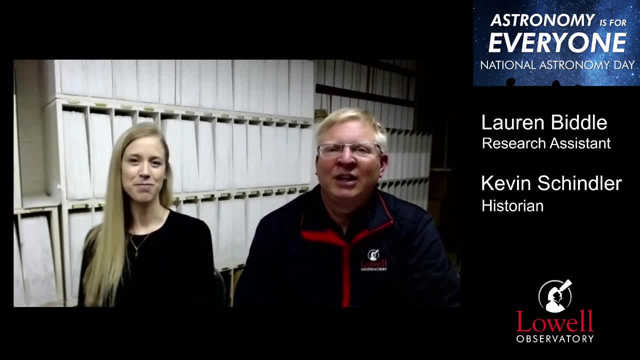 and take a look up and, really, you know, take a look at the stars and other things that are up there. It's a passion that so many people have And for some people, they become so passionate about it that they decide to do this for their career, And Lauren is an. 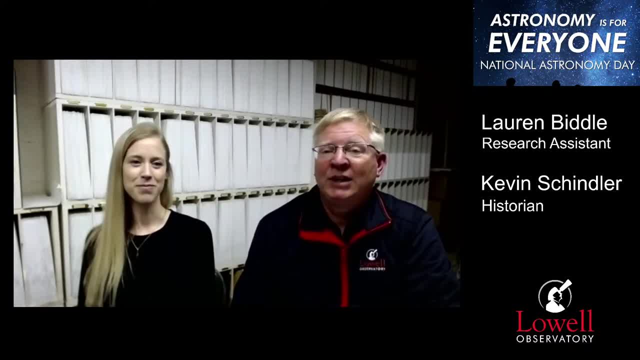 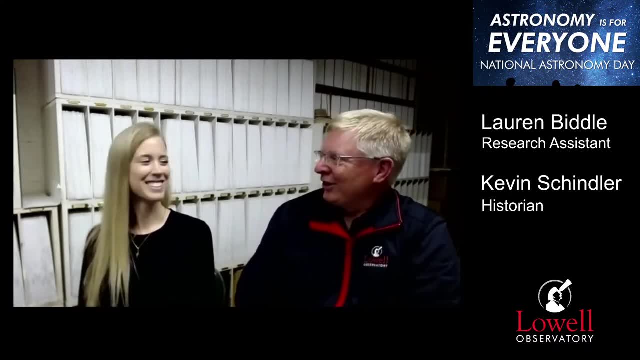 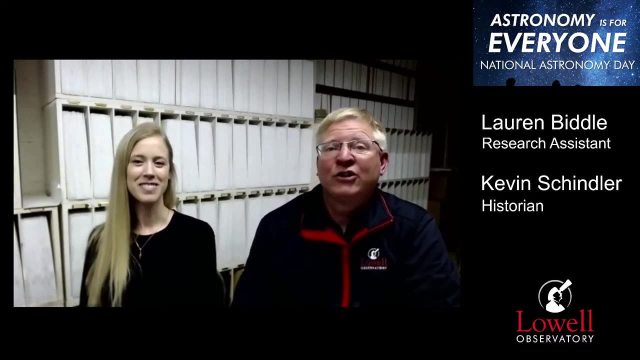 example of this Lauren is. if we do this program in another year, we'll be calling her Dr Lauren or Dr Biddle. I like Dr Lauren better. That sounds like a cool ring there because she's working on her PhD right now at Northern Arizona University while she collaborates with one. 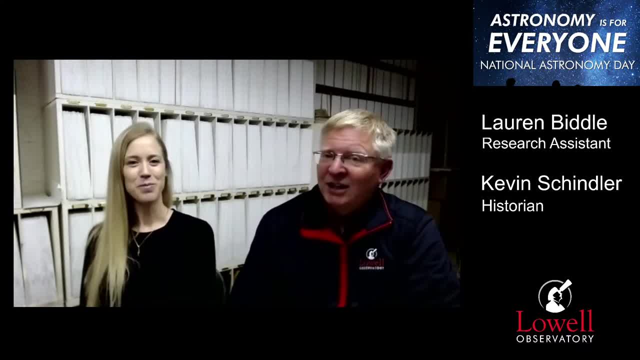 of our astronomers, Dr Lisa Prado. So, Lauren, let's just talk as we. the goal of this tonight is to talk to somebody that's really passionate about astronomy. Talk about how she got interested and the kind of work she does with the understanding. 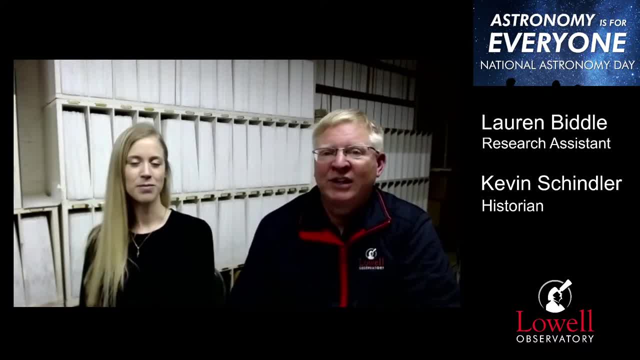 that, while Lauren is really devoted to this, astronomy is really for everybody, And we all can look up in the sky and be excited about it, And that's how Lauren started out sometime years ago. Just like so many of us, at some point she looked up and got interested. 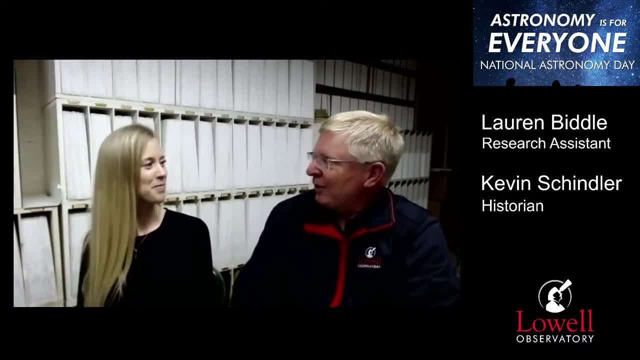 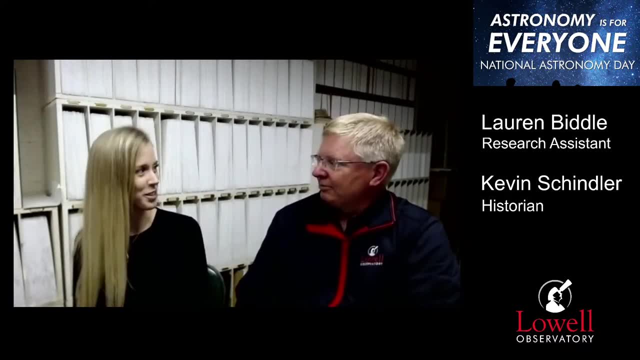 So we'll talk about that a little bit later on. But first of all let's talk about what you do here. You're a graduate research assistant, So what does that mean? So being a graduate research assistant means that you receive funding for doing research to. 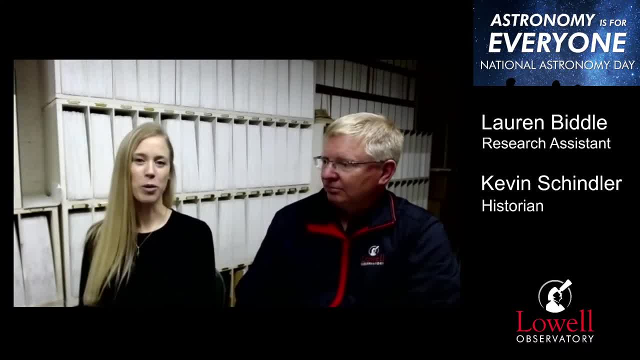 earn your PhD, And so I work with a research group here led by my advisor, Lisa Prado, and Joe Lama, And we are focused on stars and planets and disks- disks around young stars- And it's really been an amazing experience. 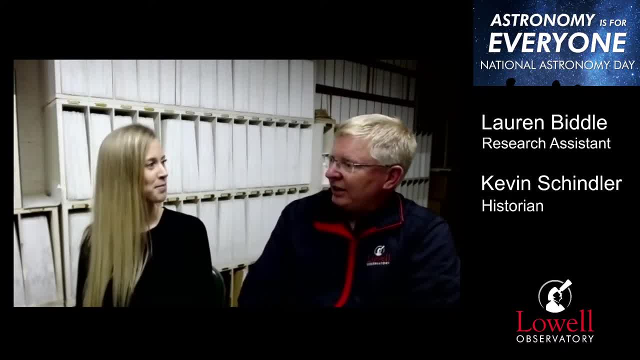 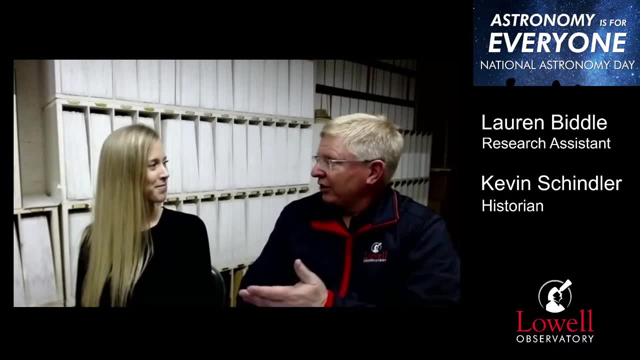 And I mean you're a graduate research assistant And a lot of people might think that as a graduate student, you're certainly doing research. You're learning how to do research, But you're not only learning how to do it. You've done some fundamental things in searching for planets around other 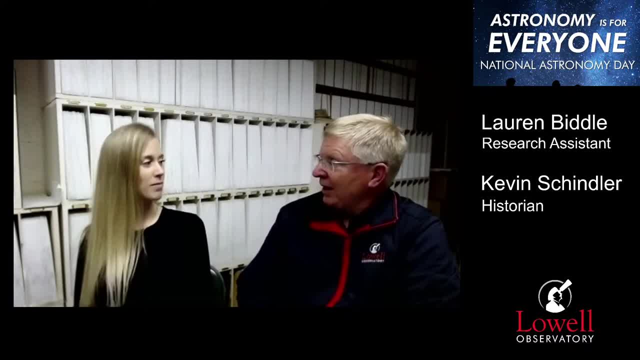 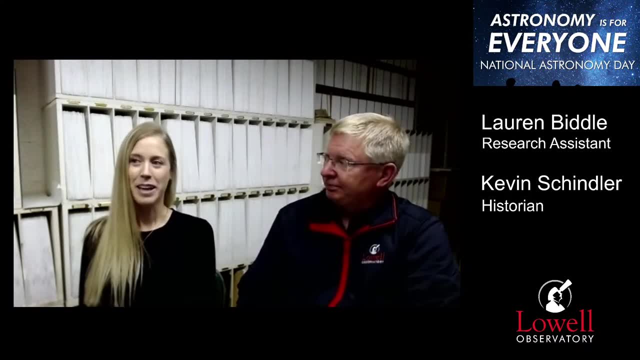 stars in terms of how to identify them Right? Can you talk about that a little bit? Yeah, So identifying planets around stars can be easier Or more difficult depending on the type of planet and the type of star, And so the type of stars that. 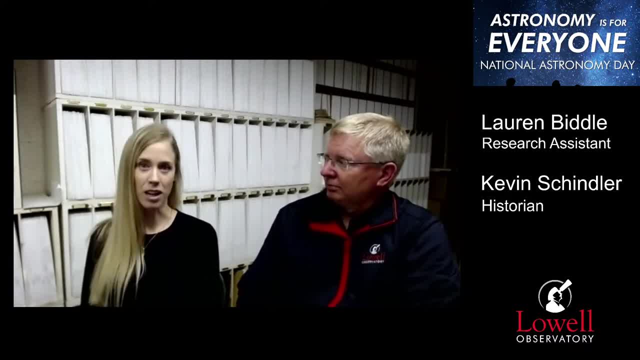 we are most interested in are extremely young. They're called T-Tari stars And these stars are only a few million years old And that might seem like a lot, But if we were to compare the lifetime of a T-Tari star to that of a human, then these stars would be like in the first week of their 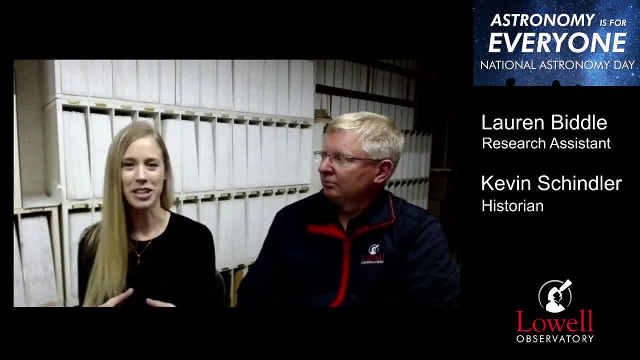 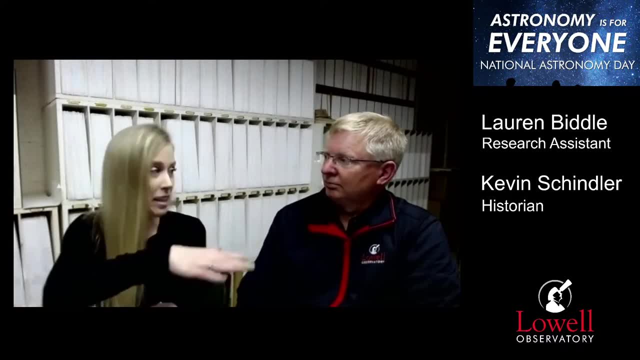 life, And so there's a lot going on here. They've got a lot of magnetic activity And they've got disks where the planets are forming around these stars, And so finding planets in those disks can be difficult. So it requires some creativity to figure out how exactly we do that. 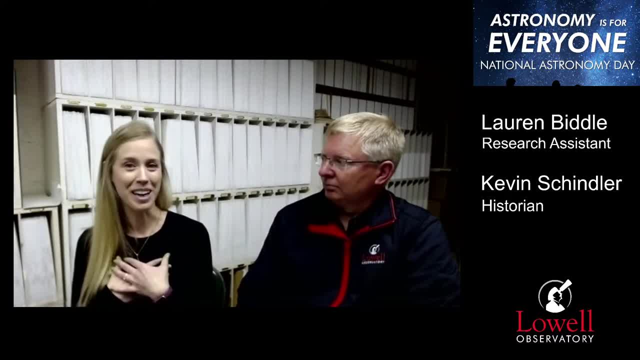 And one of the ways that I've learned that we can do that. my team and I actually developed this method And it's kind of a very interesting way of detecting planets around young stars with disks, in that the disk of the planet- my apologies, the planet- will interact with the disk And we can see. 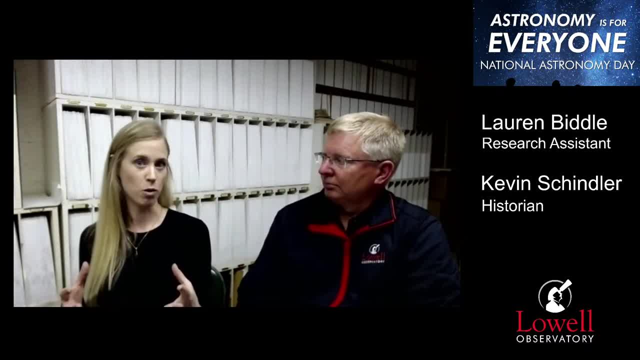 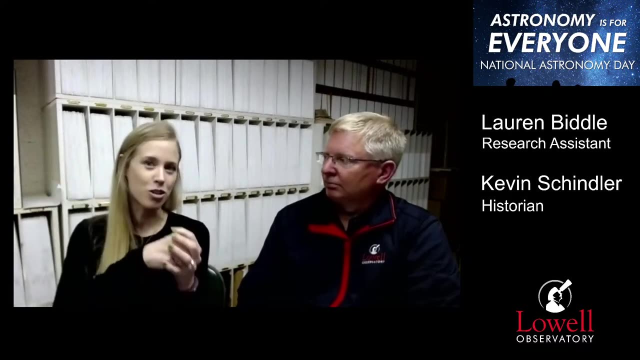 that in the, in the form of brightness changes of the system over time And in the- yeah, brightness changes of the system over time, by accretion, And what accretion is is material from the disk traveling along magnetic field lines on to the surface of the disk and then it's going to move over the disk. 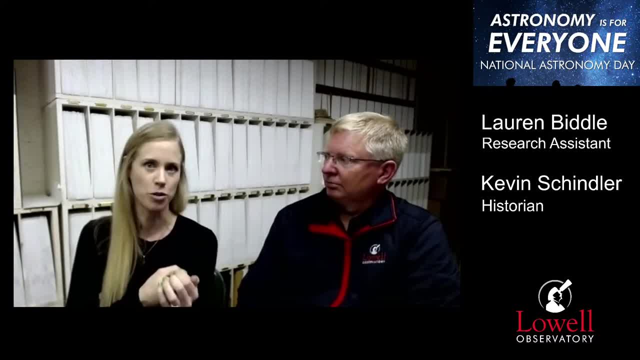 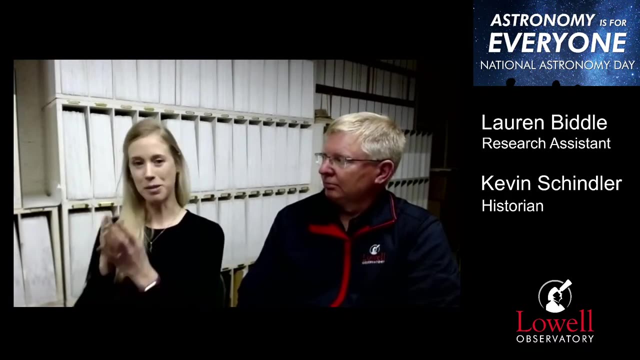 And that basically creates a huge explosion on the surface of the star, And that's what we're looking for, because the planet will pulse that material down onto the star. So really, what we're detecting is evidence that a planet is there, but not the planet itself. 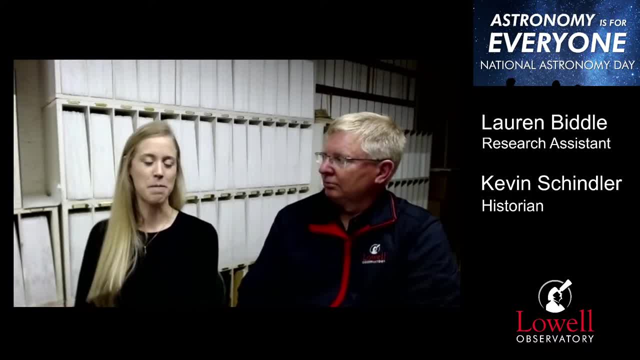 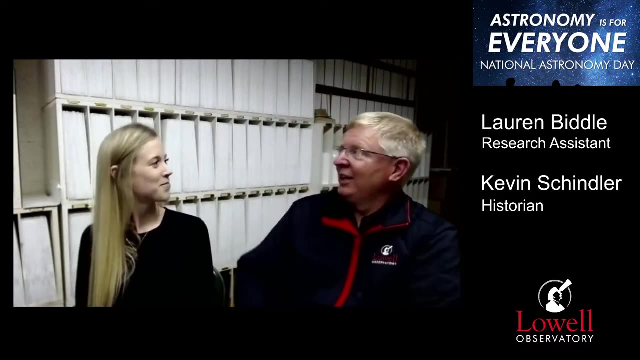 And so, because of that, it requires additional observations to confirm their existence, But this is one way that we can flag it up and say, oh, there might be a planet around this kind of star. You know, one of the reasons we decided to operate from this room, of course, is this represents a search for a planet that started more than 100 years ago and culminated in 1930.. 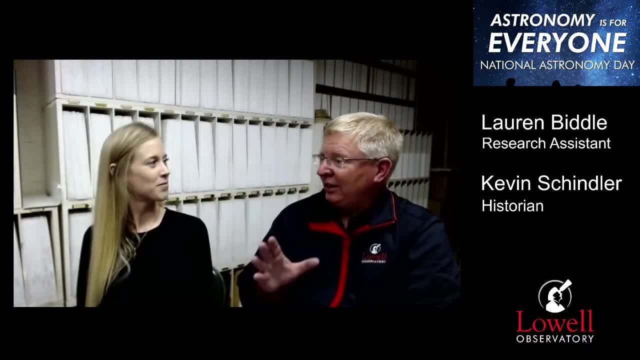 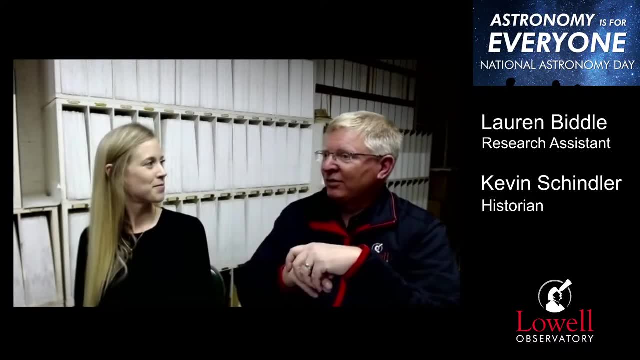 And you think about the techniques? the same thing. They didn't. They were guesstimating where to look, based on the irregular movements of Uranus, Neptune, Percival, Lowell, starting in 1905, starting in 1905. 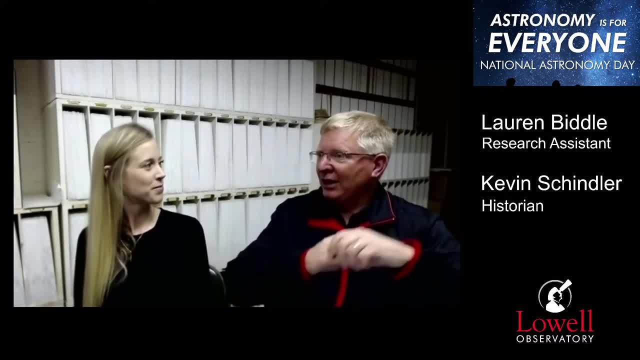 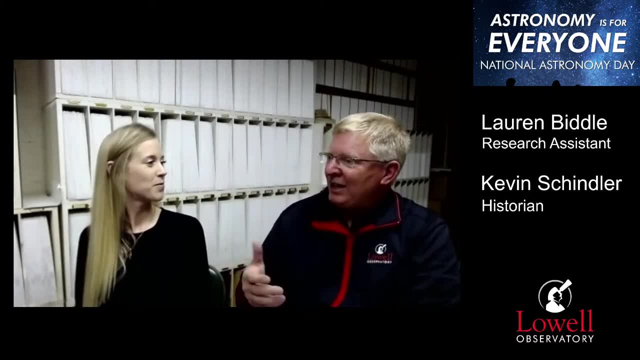 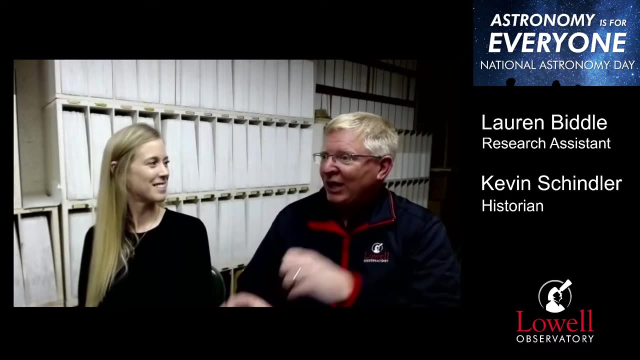 They were predicting, based on how these are moving, there should be a planet located in a certain place, a certain size, And so a lot of the same different techniques and yet the same idea of inferring what's out there, And there's a lot more to the Pluto story that this planet they were looking for. that was really big, isn't there? 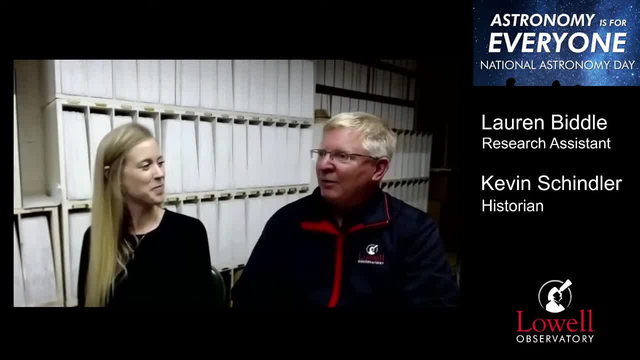 They just happened to find little Pluto right there. But that's part of the excitement of doing science is sometimes you look for something specifically And that's what we're looking for. Other times you find it, Sometimes you don't, Sometimes you just happen on something. 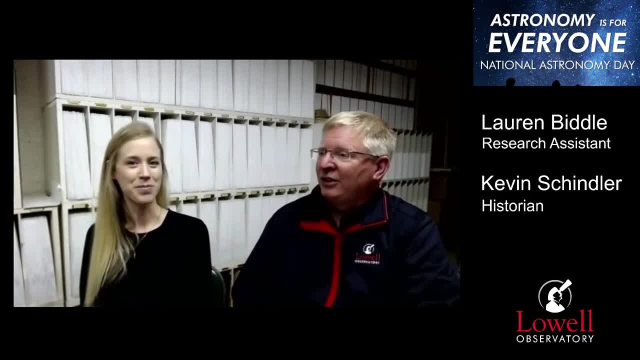 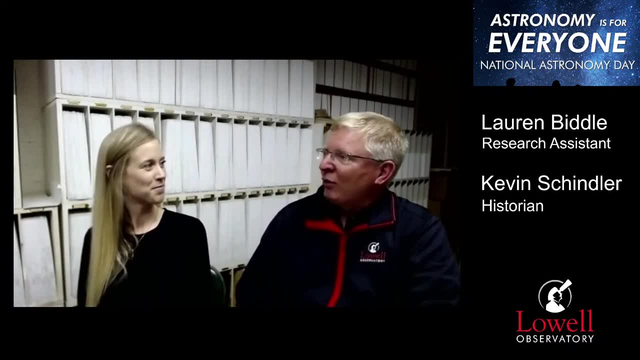 And it's just part of the process of really doing it, and doing it systematically and well, Definitely. yeah, So we've come a long ways in planetary searches. Absolutely. How did you get interested in doing this? Were you always interested in looking for planets? or, as you become a graduate student, did you have a professor that inspired you, or how did that get going? I've always been curious about how we got here, And so that question was the driving force behind my interest in exoplanets, Because I would love to find other systems that look like our own, that could potentially host life just like us, And so that was- yeah, that was mainly the driving force. 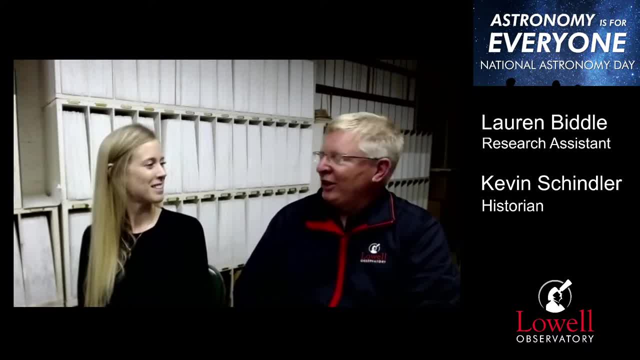 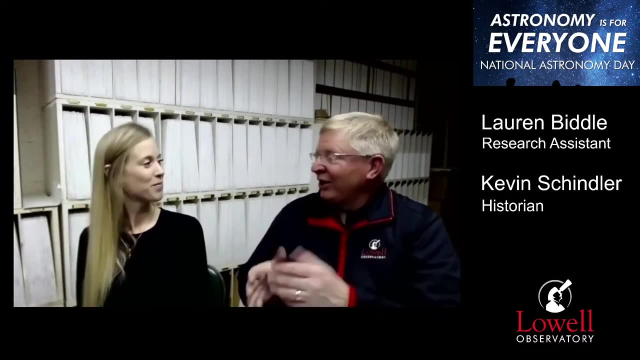 And you know it's somehow perfect that you're a low observer. You've been here since 2015, in a place where Percival Lowell, the founder, was inspired to study Mars with the idea: are we alone? That's why he started this observatory. 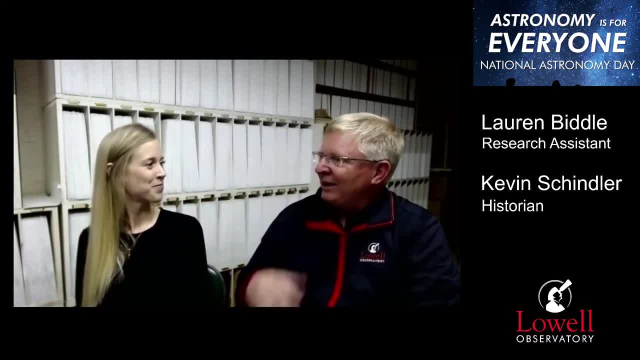 And you're continuing that mindset 125 plus years later. So it's a really neat tradition, Although the techniques you're using are a little bit more advanced than what we were doing back then. So how did you get interested in astronomy in the first place? 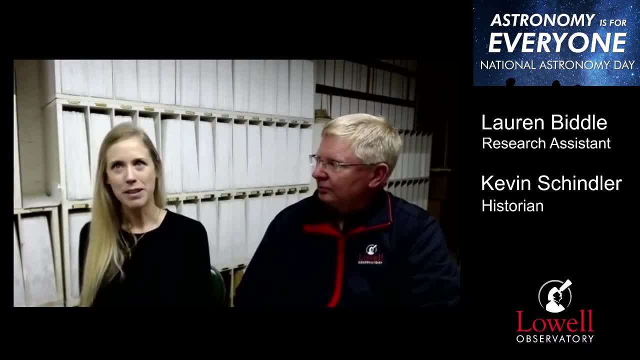 So I've always been curious about the world around me. When I was very young, I remember asking a lot of questions And at one point I think I was really frustrated that there weren't a lot of answers to the questions that I had. 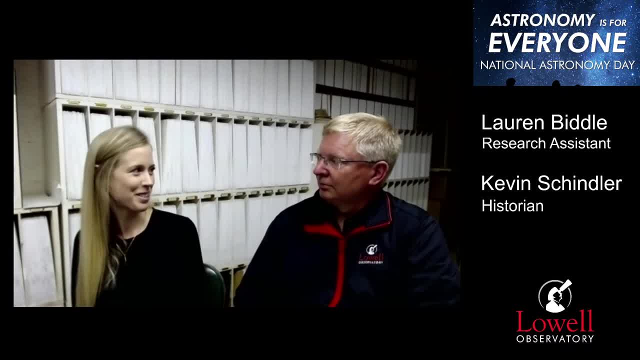 And so I asked my parents one year for Christmas for a book of answers. I just wanted to know. Unfortunately, I didn't. Unfortunately, no such book exists. No book has all the answers to everything ever. But that stuck with me just the curiosity. 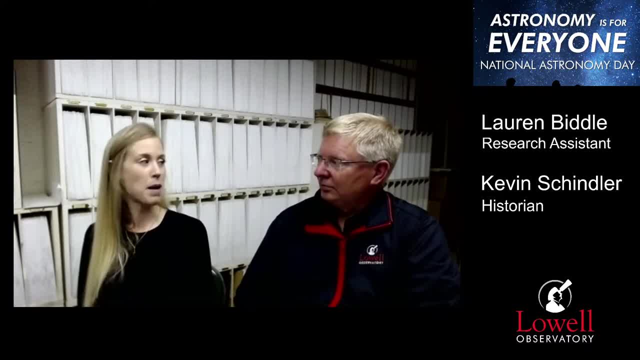 And so when I was very young, my papa, who's my grandfather on my mom's side- he gifted me a telescope And we were- they spent, my grandparents spent- a lot of time in Florida And we looked at a lunar eclipse one night through this telescope on the beach. 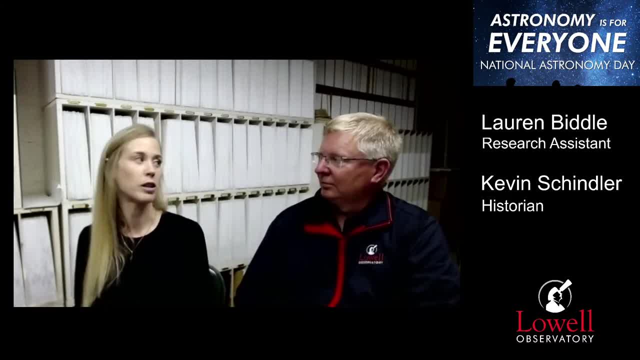 And it was like such a magical moment because there was very low light pollution there at the time And so the stars in the sky were just, it was stunning And that really that got me interested in astronomy at a very young age, And then it wasn't until I was in high school. 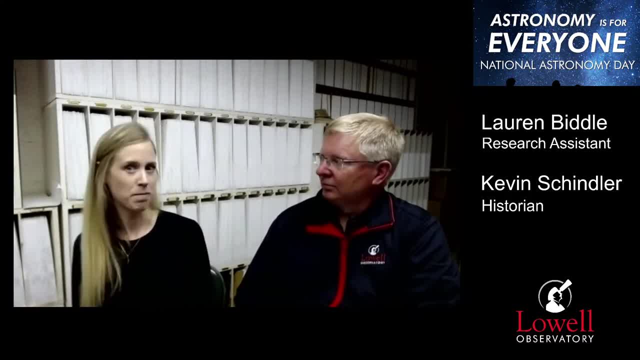 I was in high school that I knew that I wanted to do this as a profession, And I have my high school teacher, Mr Pinnell, to thank for that. He had an astronomy class that gave us the opportunity to do astrophotography. 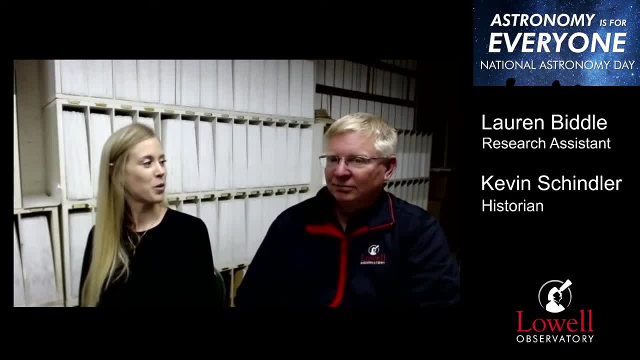 And we actually did this with film like old school film cameras, And I think they do it digitally now. Yeah, And it really just the details that go into capturing a beautiful image really, I think grabbed me And I was like, yep, this is it. 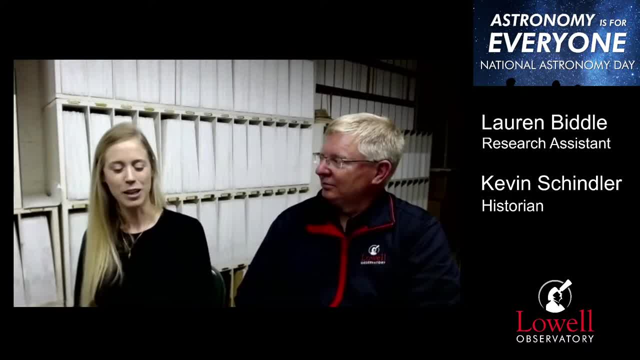 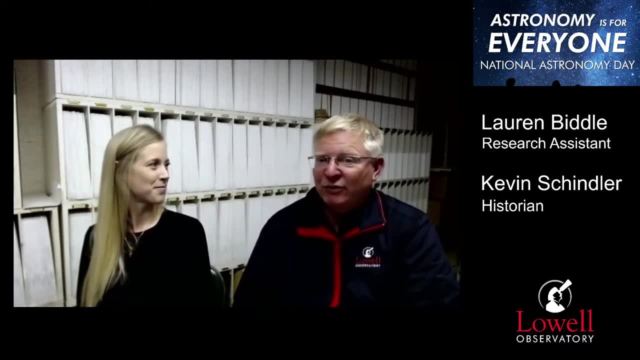 This is what I'm going to do, And so, yeah, it's kind of like my a shorter version of my journey. Well, that's excellent, And I was going to ask a follow-up, but we also have a question from David Moore. 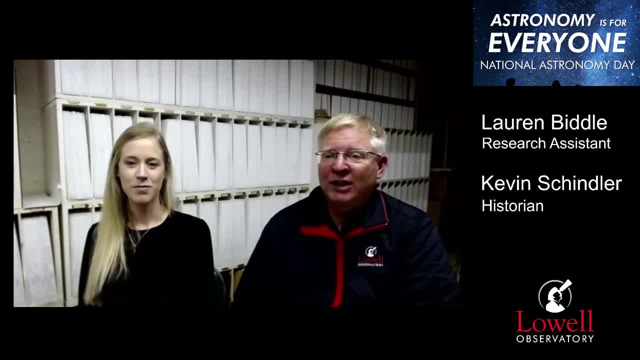 And it's a good reminder that if you have questions while you're watching for Lauren about her research- how she got interested in astronomy, anything like that- write them in and we'll try to get to them. But David has several questions. What made you choose this specific part of astronomy when there's so many different things? 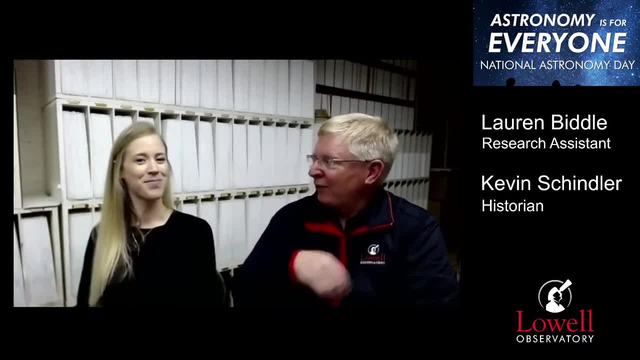 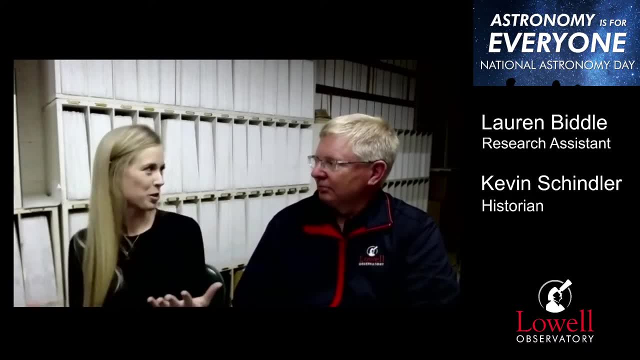 And also, which telescopes are you using? Because he lives that far from the Little Discovery Telescope. So yeah, So what made me choose this planet was just the curiosity, Just the curiosity about how we got here. And then the telescopes that I use: I do use the Little Discovery Telescope. 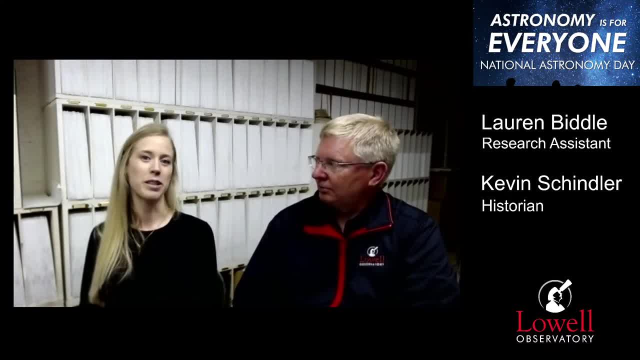 And I've also been using lately telescopes in space. There's the Kepler telescope that is currently doing the K2 mission, which is the follow-up mission to the NASA Kepler mission, And then I've also used telescope, or sorry data from TESS. 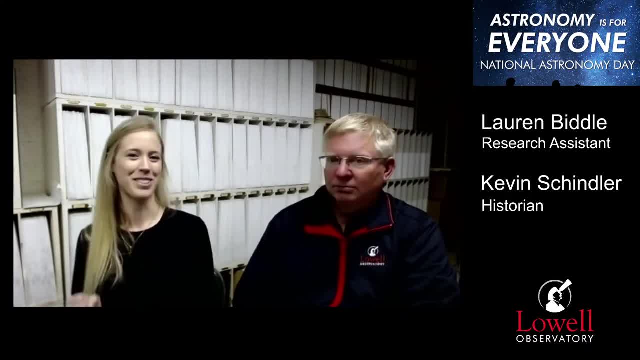 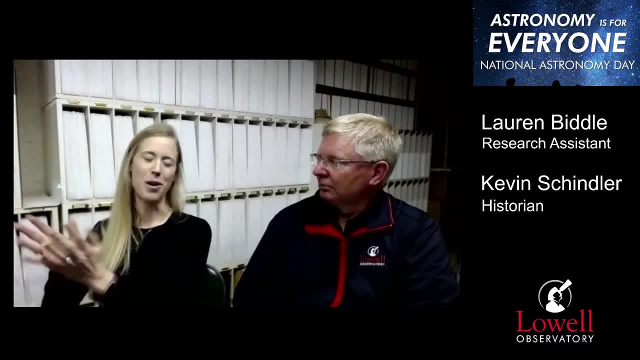 And so what this allows is we don't have to take breaks for daytime. We can just observe certain parts of the sky for all time. Well, not necessarily all time, I guess. Like for TESS, it's like 30 days in a row without any breaks, really. 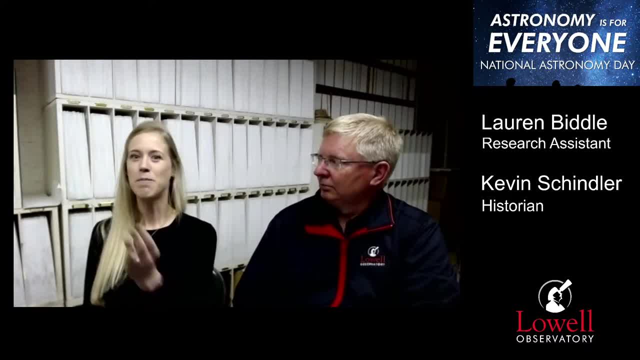 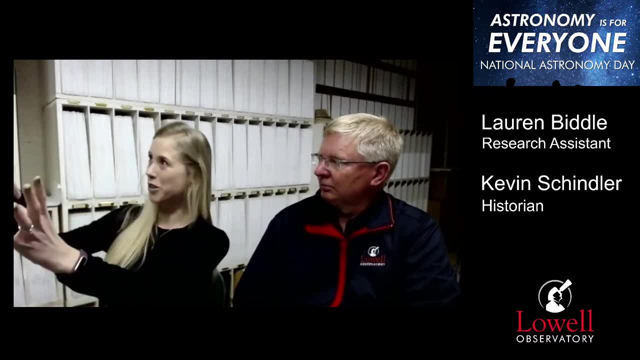 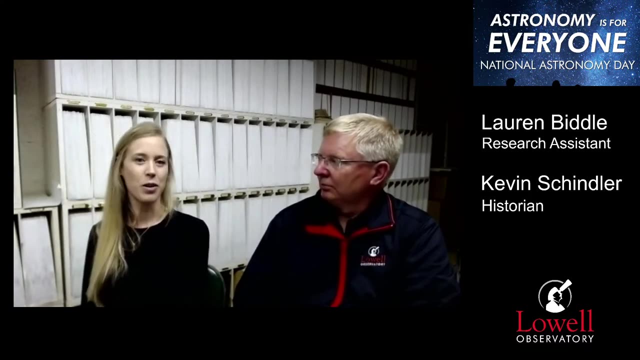 We can take data And then for the K2 mission, which is done now, we could stare at a single part of the sky for like 80 days- I think is what it was- And the Kepler mission before that it was like four years straight. 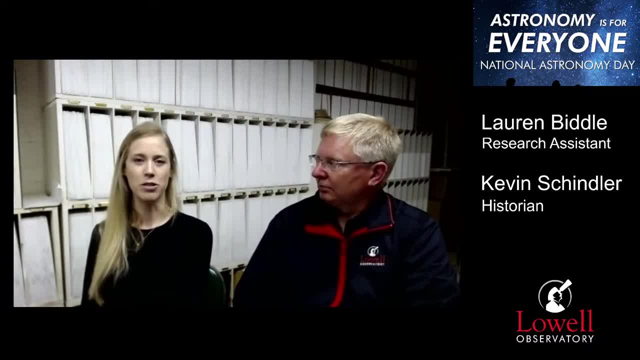 And that was so important for discovering planets around other stars, because we could detect more transits that way. And so what a transit is is when the planet passes in front of the star, in our line of sight, it will create a dip in the brightness of the star. 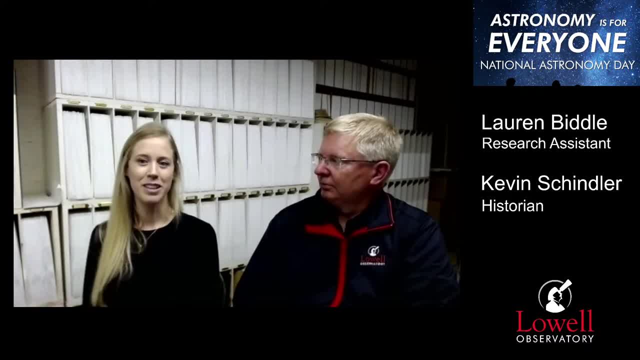 And it does that periodically as the planet orbits. So the longer we can stare at the piece of the sky where stars are, the more likely we are to catch planets that are transiting further out from their star, because it takes longer to come around and have full orbits. 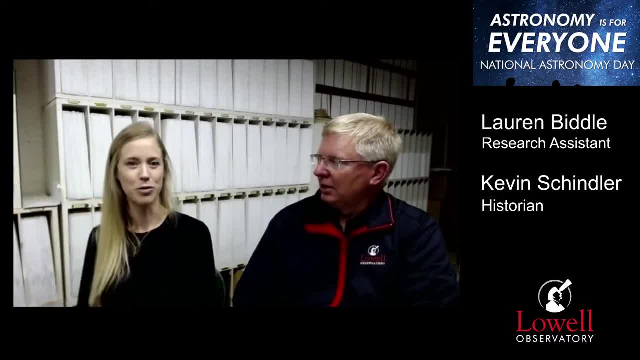 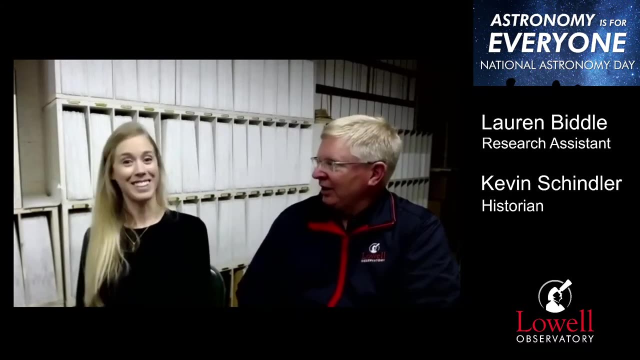 So, yeah, that was incredible for the advancement of this area of my science. Yeah, So there are several techniques for finding planets around other stars, And over the last several years, the number of known planets has skyrocketed. Is there an estimate of the percentage of stars that have planets? 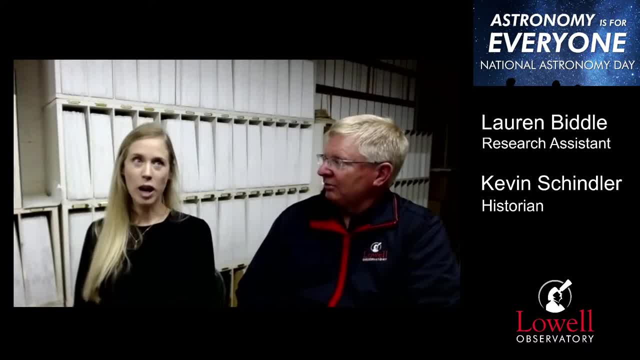 An estimate of what that would be. So there have been studies done for different types of stars And I don't remember the specific numbers right now, but it is very likely that when you look at a star it probably has a planet. Yeah, 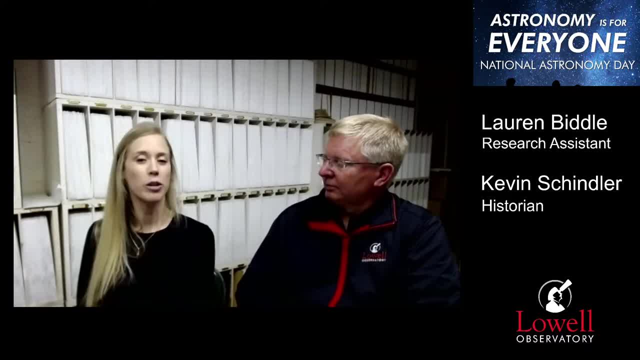 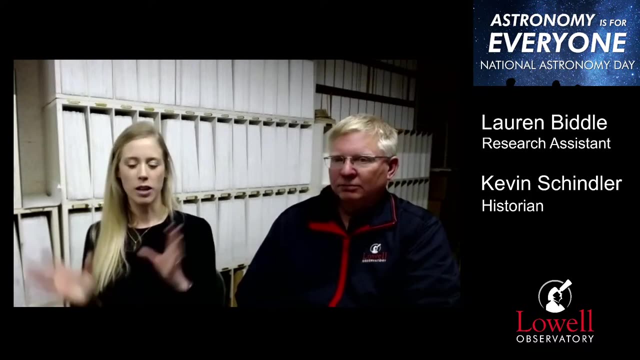 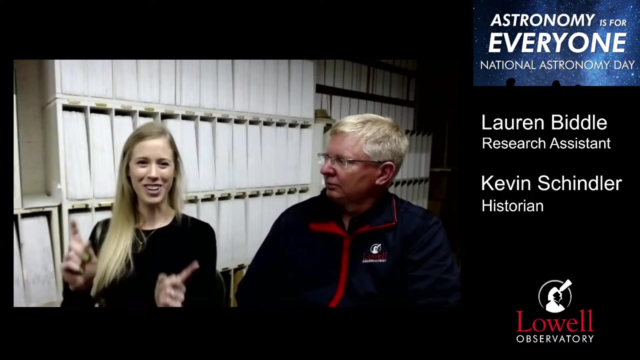 It also depends on there's current research being done on whether binary systems can have planets or like what the statistics are on those, Because even though the majority of stars that we look at are not necessarily in multiple star systems, there are enough stars in each multiple star system that, if we look at all stars, most of them are actually in binary, in tertiary and even quadruple star systems, And so multiplicity is one thing that's being taken into account currently, And so, even as we know it, the current rate of planets around stars might change depending on our findings. 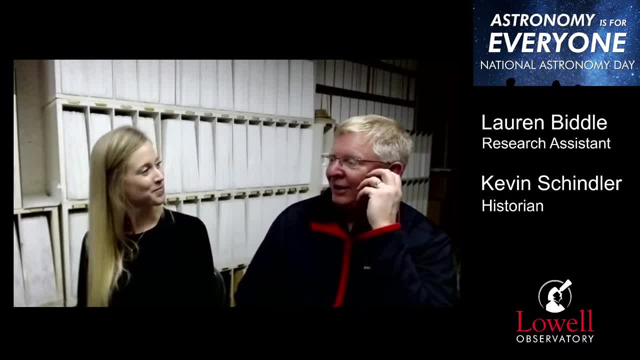 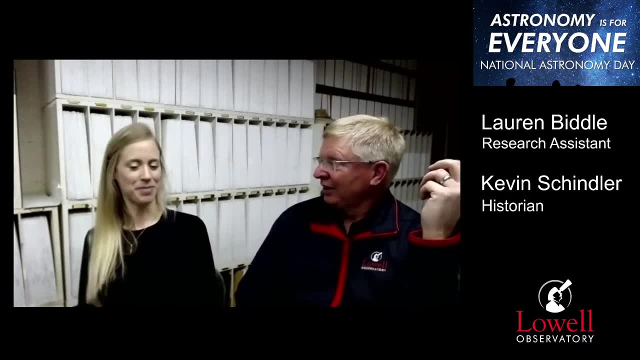 It's really fascinating to think about. you know, just fundamentally, if you're in a system that has multiple stars, you would have multiple sunrises and sunsets, And also you know what's the length of time that a planet could last with those. 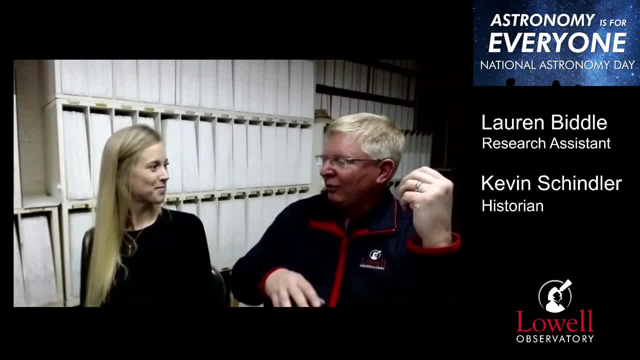 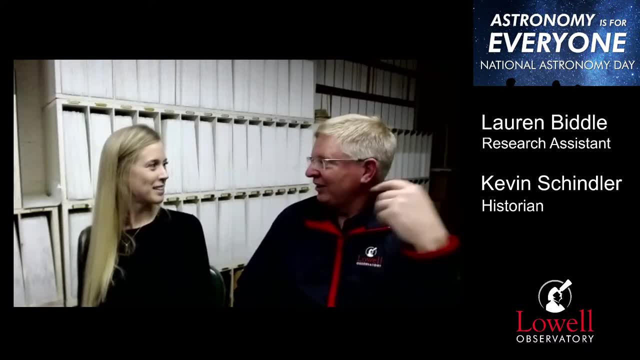 I mean the amount of time that there's regular orbiting with two, the gravity of two different stars. does it ever get to where it's stable? or does eventually, just, you know, tug apart or something like that? There's a lot to learn about it. 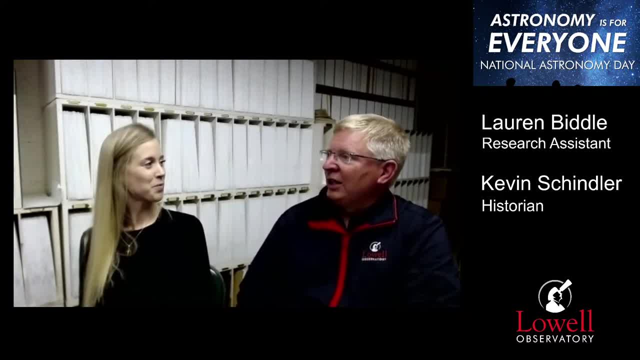 Absolutely, And so for you, you know, the ultimate thing would be to find life somewhere. Oh yes, that's the dream. So what keeps you going on a daily basis? Do you think about that every day, or is it? I mean, 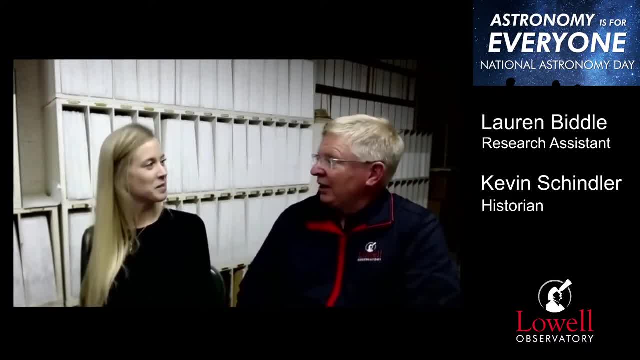 there's still the excitement of like the new method you helped develop or developed in searching for them. I mean, what keeps you going on a regular basis? Because you're. we'll talk about this in a couple of minutes, but you know. 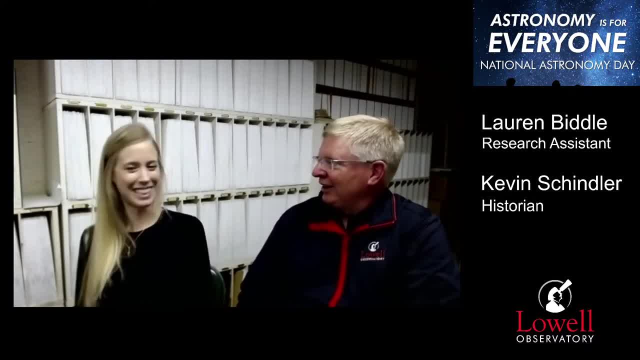 a typical day for you is probably a lot of staring at a computer screen, And somewhere along the way you kind of get tired of that. probably The eyes do. Yeah. What keeps you going on a daily basis? It really is the. 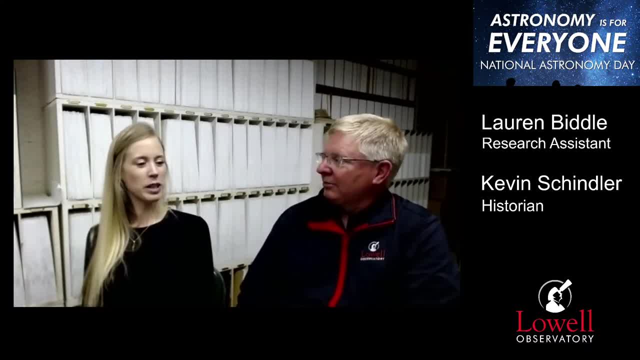 the wonder that I have, for are we alone or not? And although I may not be right now, looking at planets that are likely to host life, remember these planets are extremely young, So they're probably, you know, they're still forming. 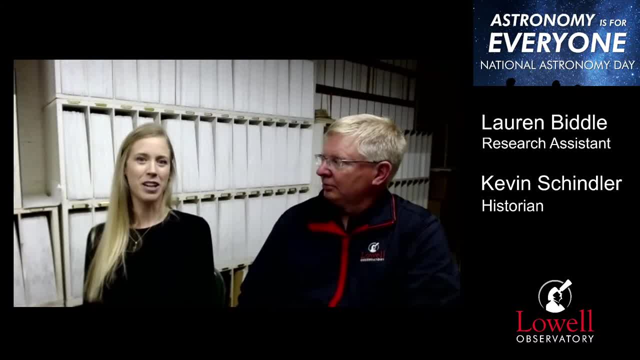 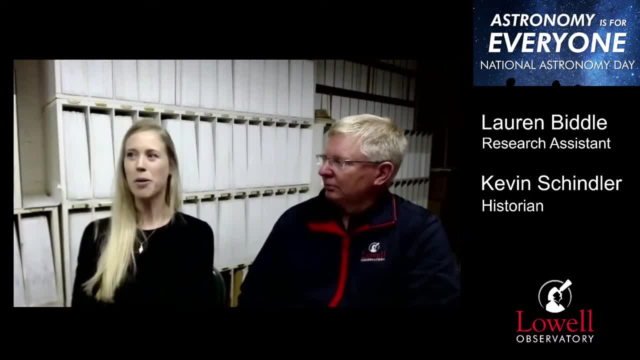 it's, it's, it's, it's, it's not not suitable to host life right now, but those planets might someday be, And then that can help inform our searches for life Now. And so it's, it's like. 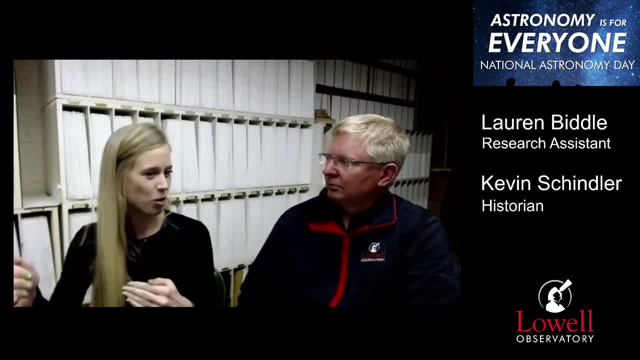 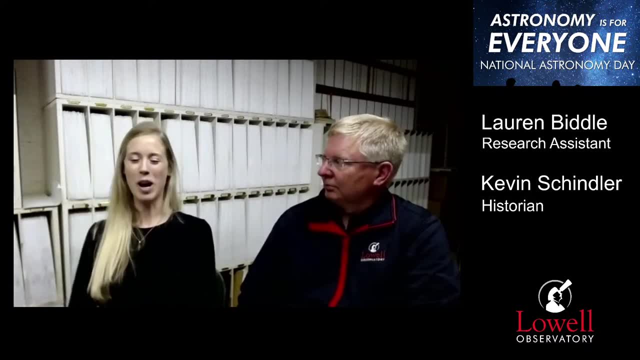 okay, so what can we do to get to the end goal? And then, even at the end goal, like, we will have more questions? That's one of the things that also I've found is that the more answers we find, the more questions we have. 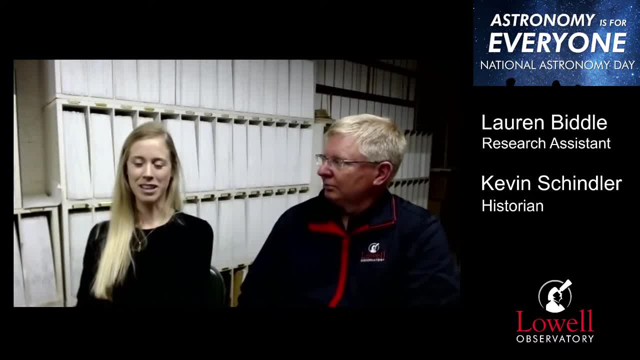 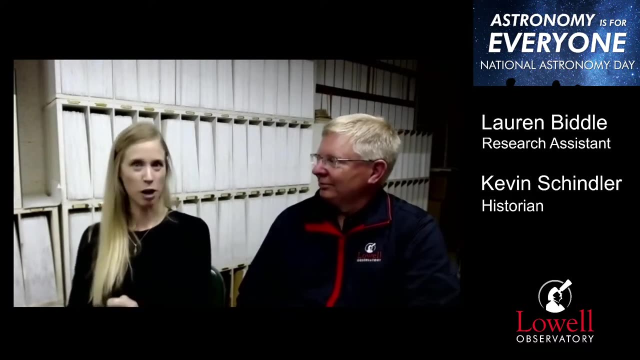 And that is just one of the things that keeps me going or just doing: 가르� Wieder Buds foreign. just the more questions I have. and then sometimes I'll just like lay awake at night and I'll just like have an idea come to me and I'm like, oh, I can't wait to get up and try that and like test. 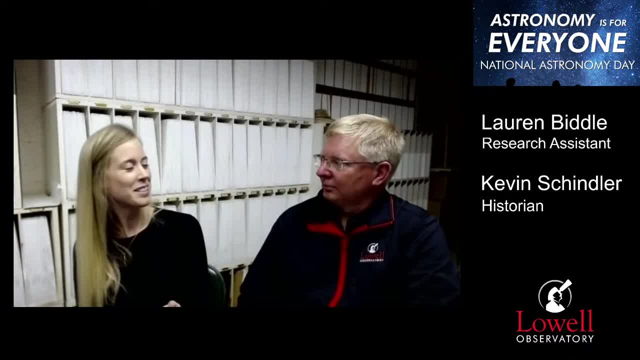 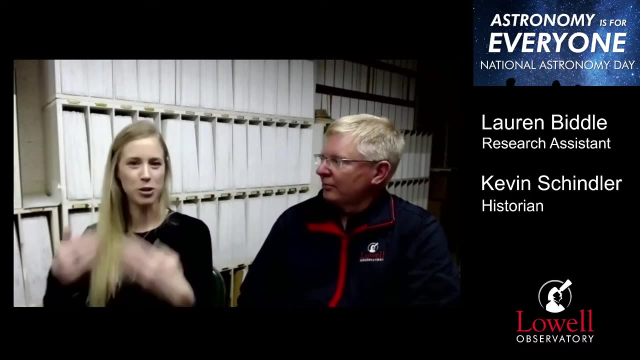 out my hypothesis, and sometimes it works out, sometimes it doesn't, and when it doesn't it's. it's not too discouraging, actually, it's just part of it, and sometimes those will even spur new ideas, so it's just like a self-perpetuating machine. that's how science works. yeah, keep. 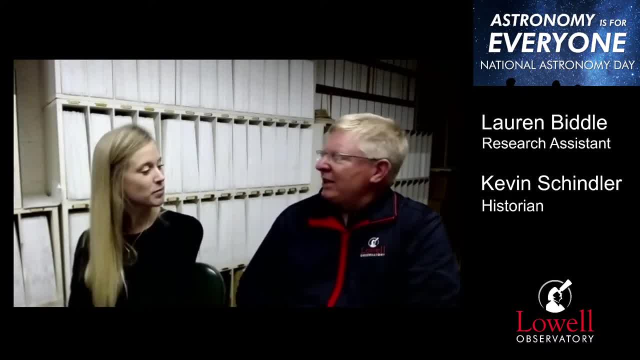 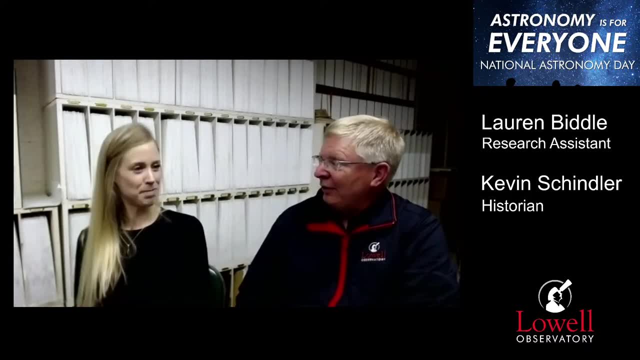 questioning: um, so what's a typical day look like for you graduate students? I mean, you're also affiliated with Lowell Observatory here. um, so do you have a typical day? yeah, so, um, as the the current stage in my graduate career is the stage where I don't have to take classes anymore, and so 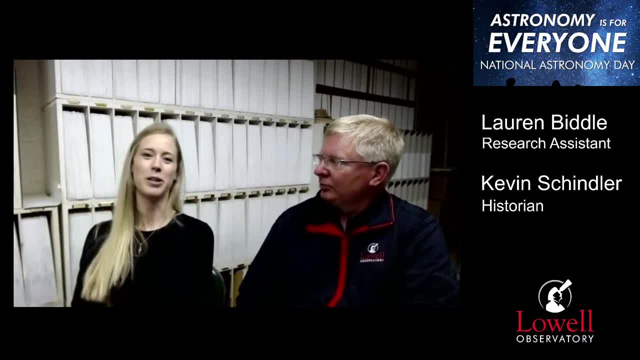 earlier, maybe like the first two to three years, I would take classes on like planetary systems and formation and how that might come about, and so that really lays the groundwork for what I do now, which is I'm done with classes but I still get research credit and um, so I will. 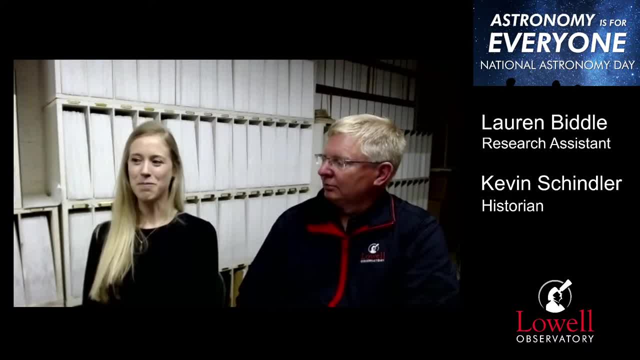 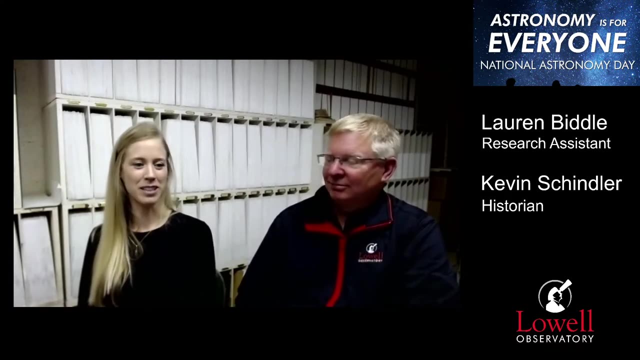 wake up and I will- um, I mean honestly just like get on my computer and get going, but, uh, with some caffeine helps, you know, you're powered by coffee, but um, but in all seriousness, it really is a um it's. there is a lot of coding involved, so I I write a lot of um coding or scripts in. 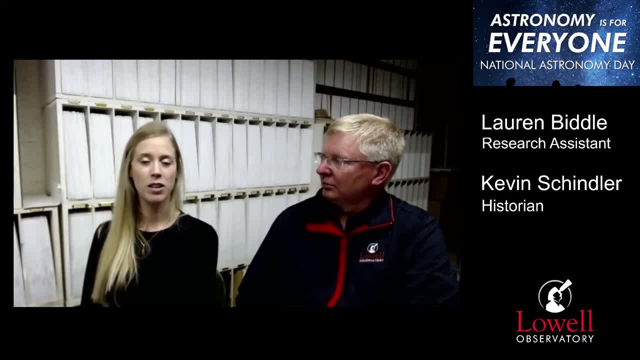 Python to help do some analysis on what I'm doing. so there's a lot of statistics knowledge that I learn and, um, some of it I actually have deep and learned in my classes and that requires me to have some like self-directed learning there. so like, where where could I go? who do I talk to to learn more about Bayesian analysis or something? 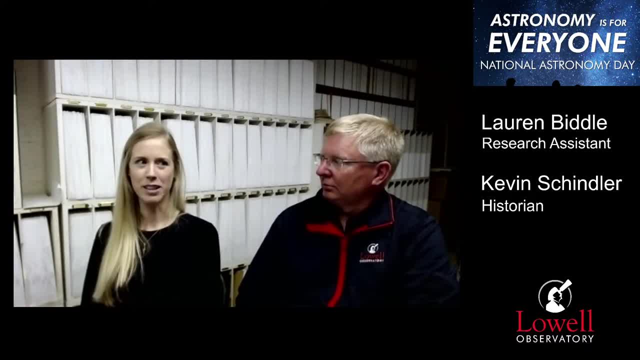 like that. that's just um, a way to calculate, uh, more informed probabilities, and so, um, some, a lot of it is teaching myself things and, um, yeah, lately I've been working from home, um, and I have teachers there who cheer me on, and so I'll go over and I'll say hi to my guinea pigs and I'll 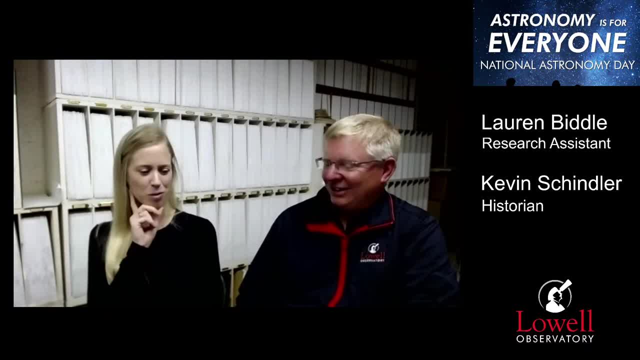 ask them questions like: so what do you think about this result that I've found? and you know, they just look at me and say: can I have a carrot? and what are their names? do they have nerd names? or uh, one of their? actually, one is hero and it's spelled h-i-r-o. hero, um, and then one is pasta. 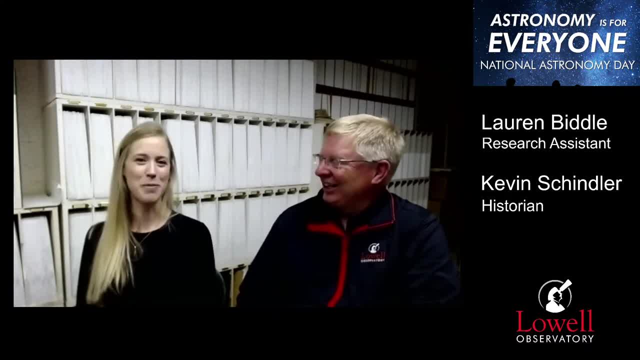 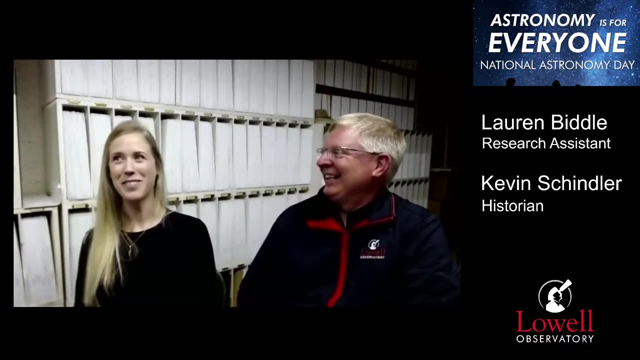 and they're. they're really sweet. keep me company. so you're a year away from your PhD. um, you're saying that with. you've said that with a little hesitancy. yeah, let's try. you're a year away from your PhD. I am. yeah, that's a little more confident. it's just, it's crazy because it's been 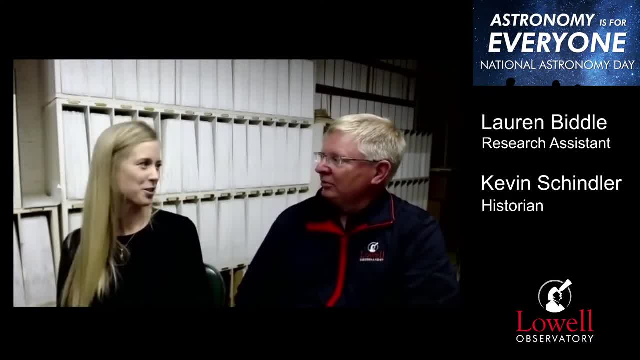 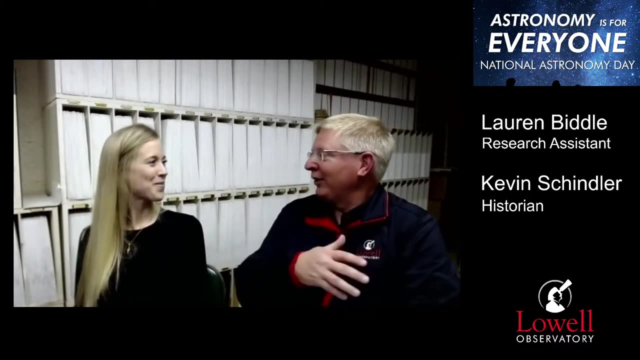 such a long journey that it doesn't feel real yet, but it like does at the same time. well, now, I mean, you have the benefit of experience, and so now you're a mentor to, you know, younger kids, um, and so, looking back, you know, when you're back, when you're five or seven, you know that's a golden age. 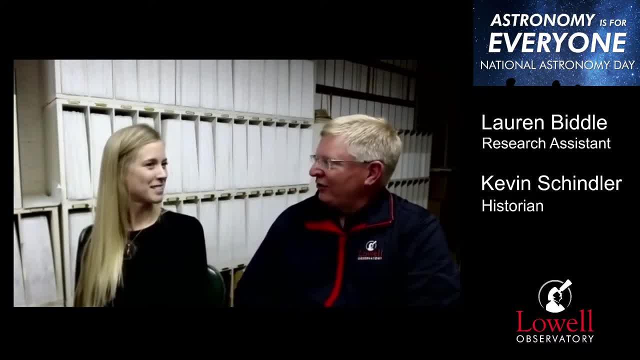 years old, you get really interested in stuff. um, what advice do you have for kids that age? you know, with your experience of having, you know, been inspired to do this, you went into it, got an undergraduate, working on the PhD. um caffeining your way through it, I mean, what kind of things? 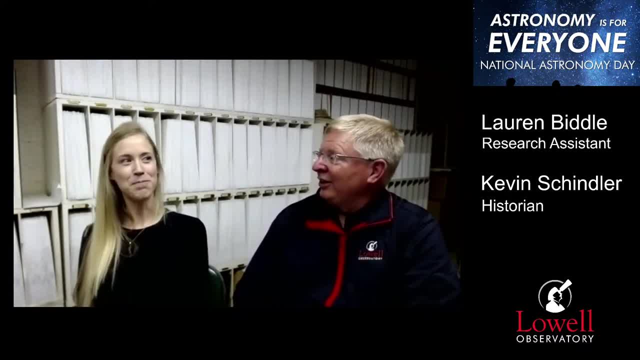 in school should you pay attention to or you know. just in general, I would say that, um, you don't have to be good at math to be good at science. science, I think Carl Sagan said this: science is a way of thinking more than it is body of knowledge. 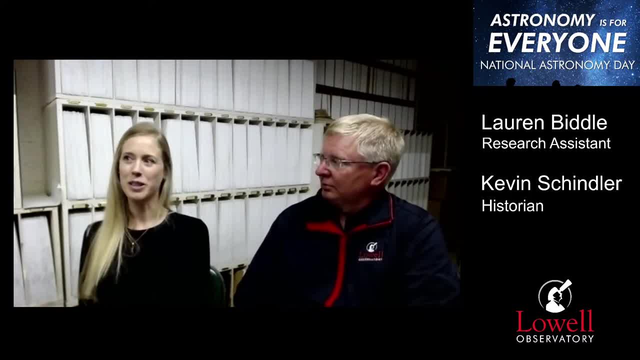 and uh, just keep wondering, keep asking questions, and it's normal if there are times where you may doubt yourself and your abilities, because this is something that can be very difficult, and um, but you can do it, you really can. there have been many times where I've had to remind myself I can do it. and um, the guinea pigs. 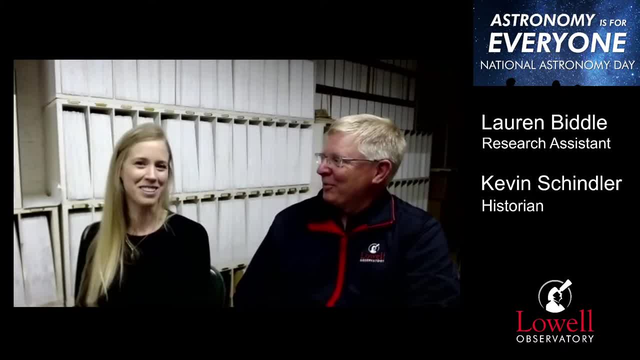 the guinea pigs will just cheer me on. yeah, as long as I give them carrots. that's the thing. yeah, that's an easy one. yeah, no matter what, yeah, questions you're asking. you know that's a certain thing: give them carrots, they'll be happy. so, um, I think we got another question here. it. 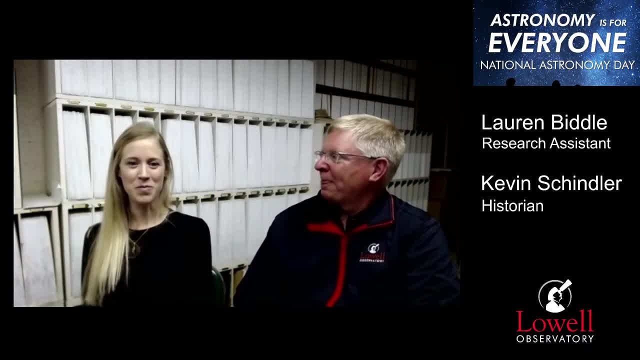 looks like when you finish your PhD. what's your dream job? well, uh, I'm currently applying for postdoctoral positions, and so I get to work at another institution with another mentor on a project that I design, and that is, that's my, my dream. next step? and, uh, just continue down the 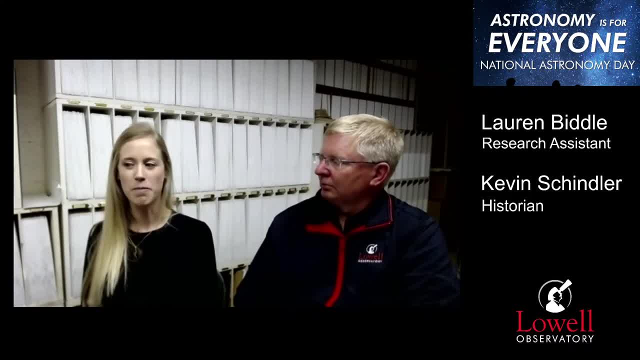 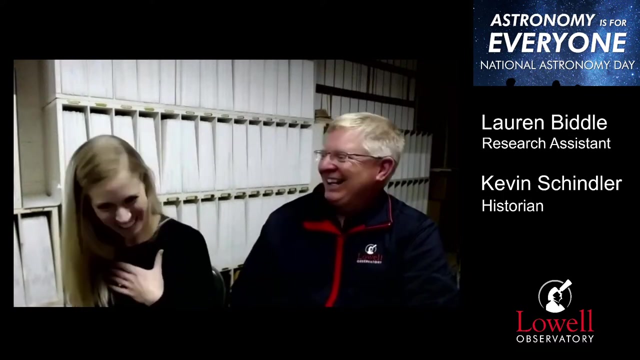 academic path by really um having the ability to design my research and um be at the forefront of human knowledge. I think is really what I aspire to continue doing. yeah, you didn't say anything about a little observatory there. like your dream job would be to be involved forever, right, honestly, yeah, yeah, it is. 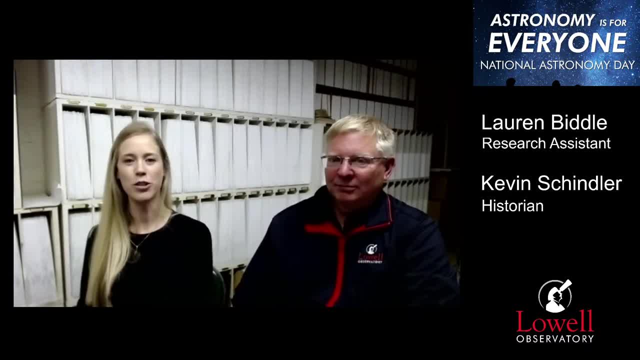 encouraged uh during this stage in my career to um expand uh out and form collaborations at multiple institutions, but I really really am thankful and eternally grateful for the support that Lowell Observatory has provided me and the resources as well. it's um everyone here really is. 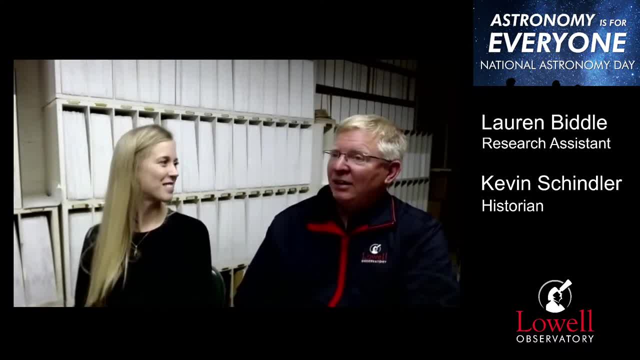 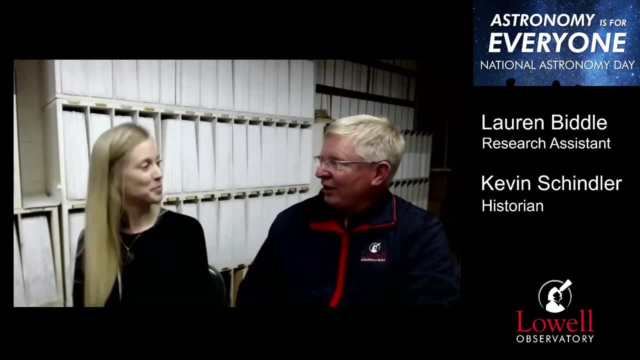 a family. yeah, it really is that atmosphere and it's. it's neat. I've been here long enough to see students come through but then later on get postdocs and get a full-time position somewhere, and somewhere down the road you know you're collaborating back with Lowell people or NAU. 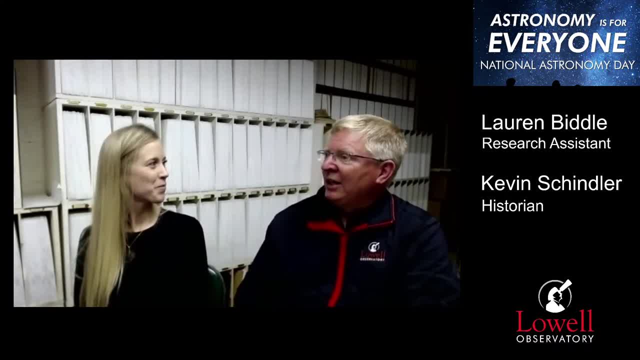 people and it's it's really a community. um, and I at least to to another question: um, you know the partnerships that you form, the you were talking about your team when you're an astronomer. I mean, there are some astronomers still that work alone and do their own thing, but in 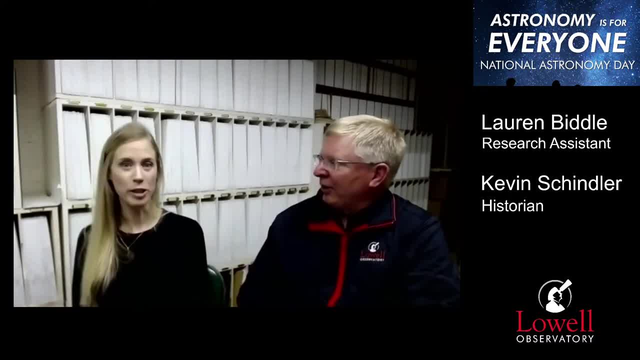 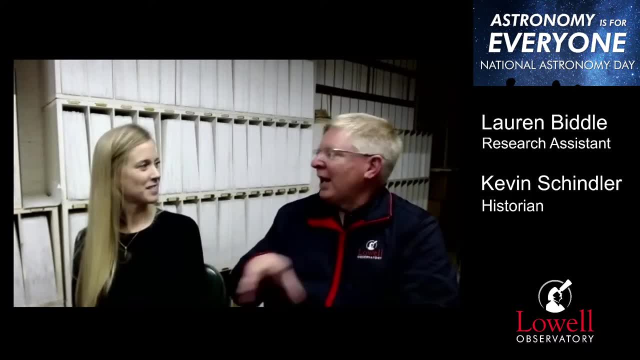 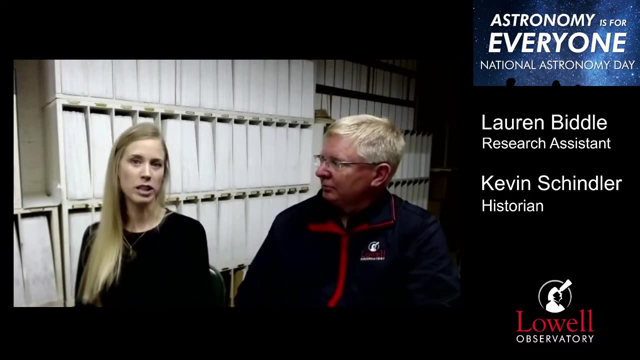 general, it's more of a team-oriented thing. maybe you could talk about that a little bit and how your team- you know here, both at NAU and at Lowell Observatory, how your teams collaborate together. oh, totally yeah. so, um, a large part of what we do is collaborative. everybody has a unique set of 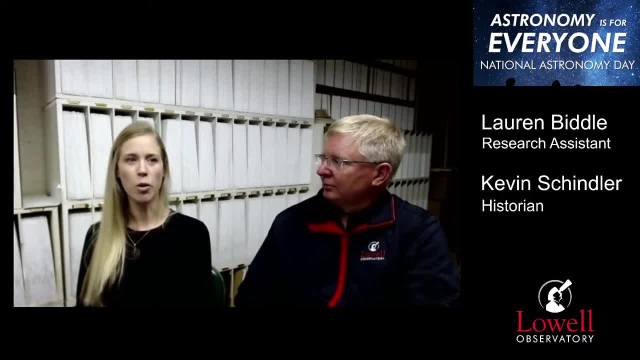 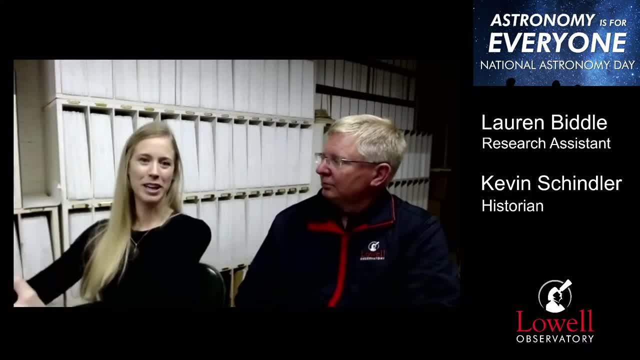 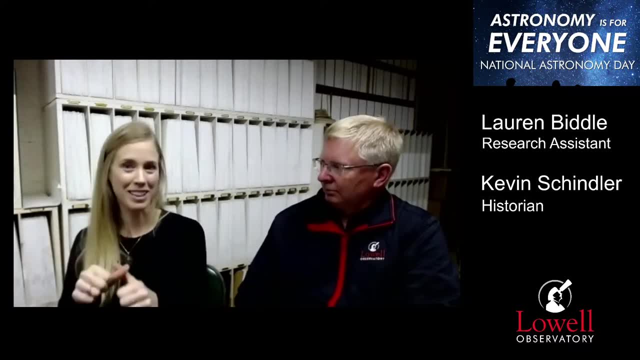 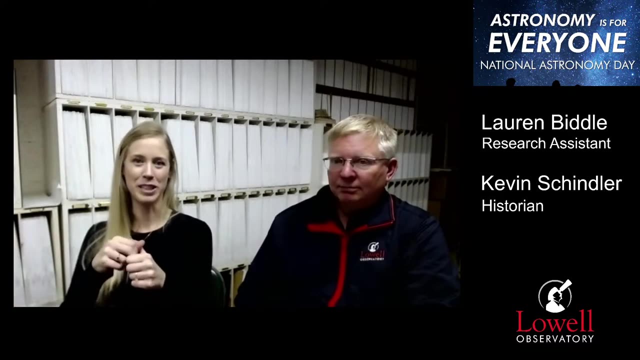 star clusters, and if they joined our group, we could discuss how our topics of interest intersect and what skills can we use to bring together to learn something that we- that only we- can do, and so one person might have a really deep understanding of like star clusters, and if they joined our group, we could discuss how our topics of interest intersect. 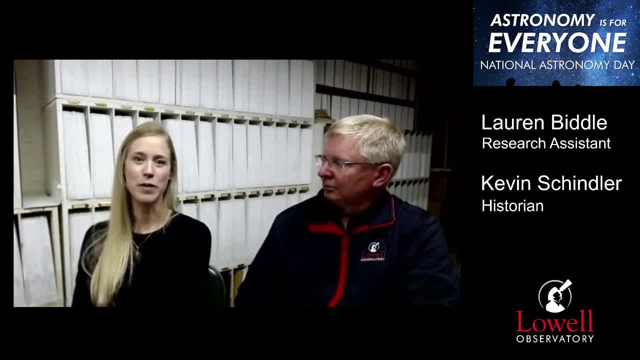 that knowledge and background that no one else does, and so and that makes every team member valuable when it in our, in our, research endeavors. yeah, and let's talk about data a little bit. we have one of our um viewers asking about, um, the kind of data, um data science that you use, because it's certainly 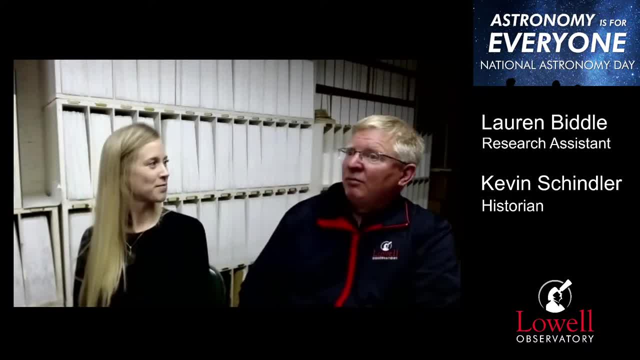 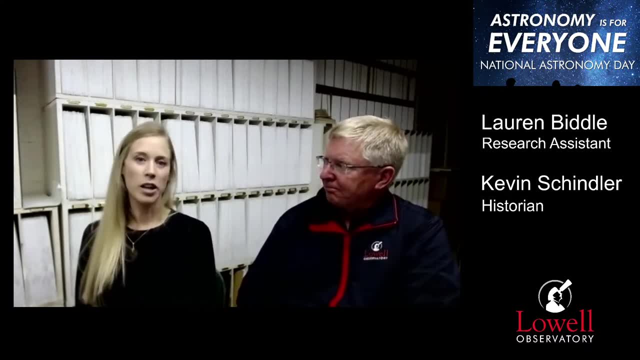 a lot different than what's behind us, um, how they both look for it, collect it and then analyze it. so maybe you can talk about that a little bit. so a lot of the data science that, um, i've had experience using and that i've seen used also. 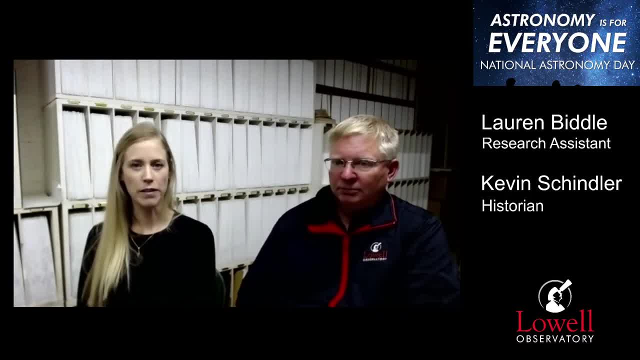 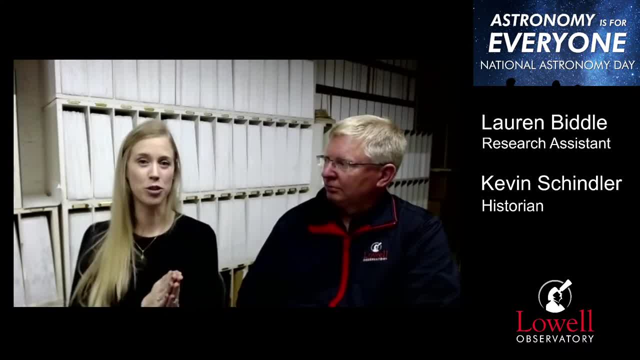 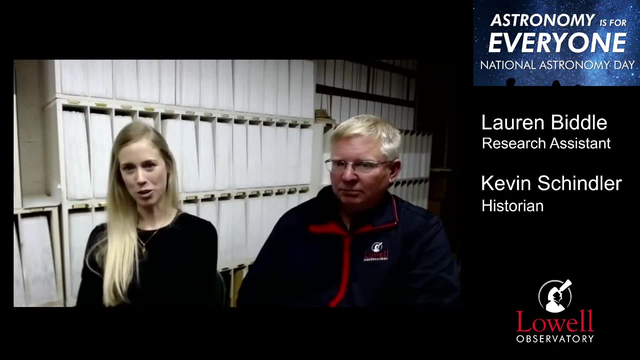 depending on how well it describes the situation that we're trying to model, then it will head toward the right answer or an answer that best fits what we're seeing, and so that's one technique that is used commonly. um, in terms of like data science, there's- uh, i have not used- machine learning- 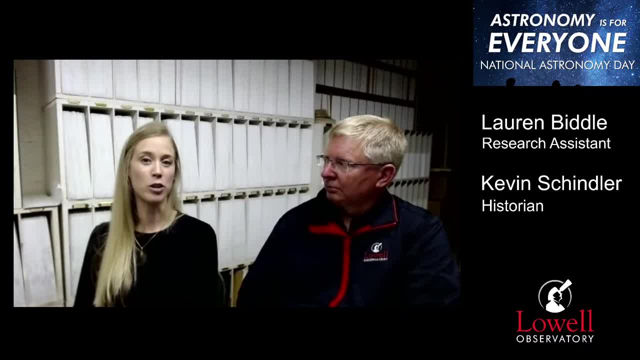 in my research, but that has become an extremely useful tool in astronomy in general, and i think it's really useful in general because we are in an age of human history, i think- where we are amassing so much data and uh, there are, there are even some next generation telescopes that will come online. 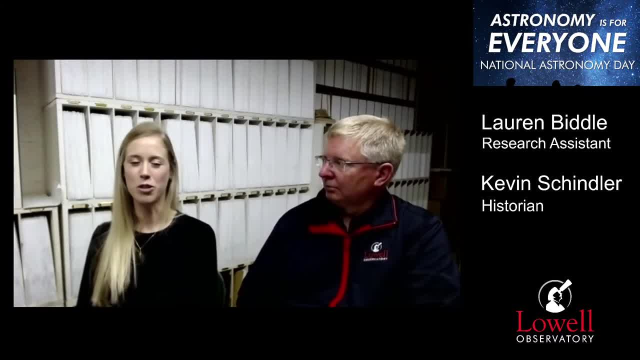 like the lsst that's going to require data science, to the point where we'll probably be utilizing techniques that we haven't even thought of yet. um, yeah, that's just just a few, and you know it brings up something, because you're you know, we're celebrating national. 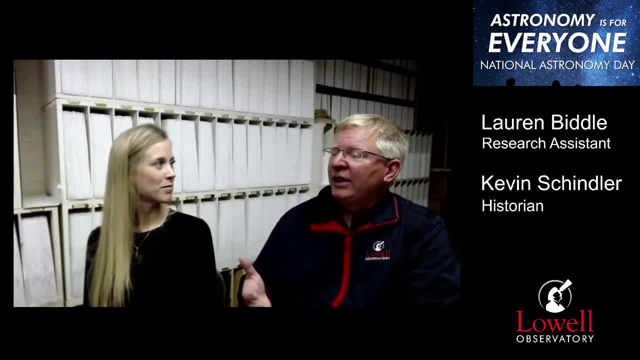 astronomy day and and really you know we. one of the key things we do here at the observatory is make space accessible for everybody. so we, from the beginning we carry out cutting edge research, but we also make it accessible um and fun for people where you can come up and look through. 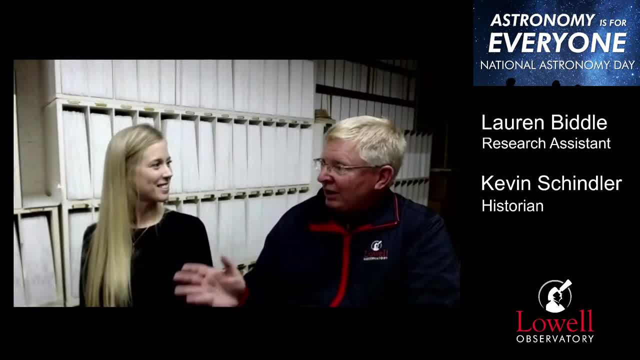 telescopes. so it's neat because you're- you're, you know, like you know, kind of the typical low person where you're really critical. um of all know, and i think the challenge is more that in excited about your research and can start nerding out but but on the other hand you don't have to do. 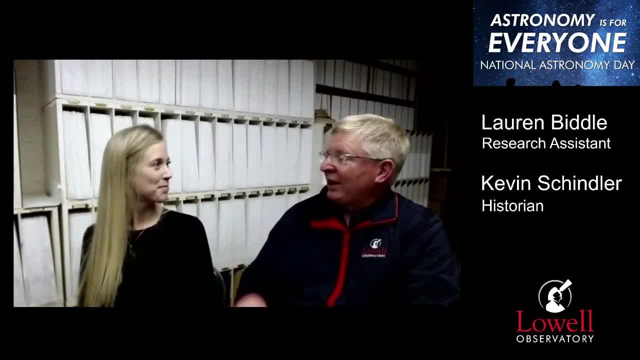 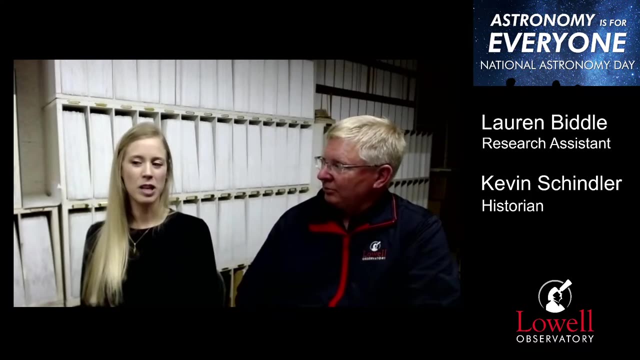 that to appreciate the nice guy. i mean what? what do you do besides, when you're, you know you're looking at the numbers and everything. what else do you like about astronomy? that's just, you don't need any training or anything. anybody can do it. yes, that is so true. um, i love that i can especially. 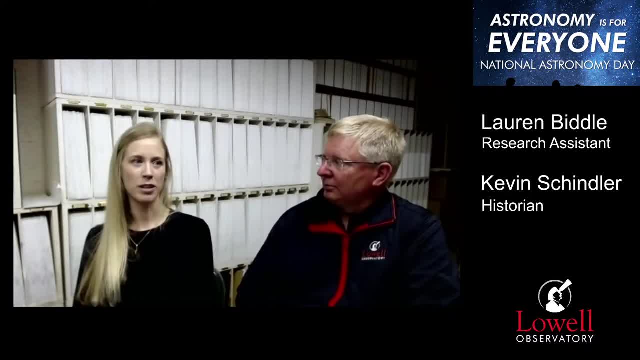 in in flagstaff. i love that i can go outside and we're in a dark sky town right there. the, the lights here are designed for, uh, the ability for astronomers to see the night sky better, and so, um, i like that i can go outside and then remind myself that the the data i'm seeing on the screen. 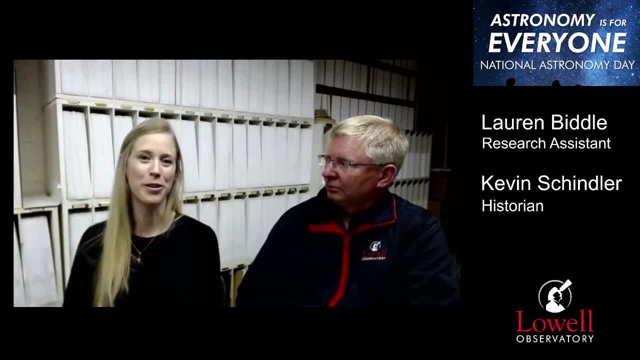 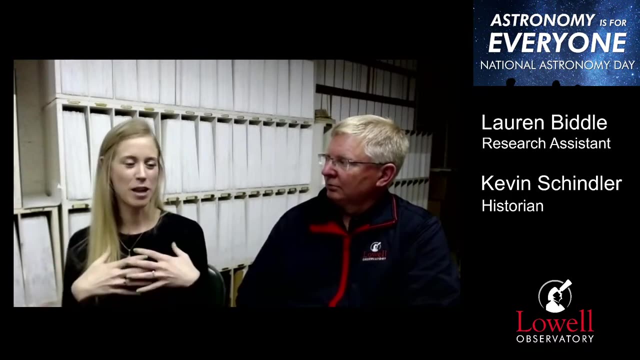 is very real and i am as much a part of it as it is of me, and it gives me more um human context, like where, where i exist in the universe and my family and friends and the world, and how, the how does this fit? and i think that's that's what i like about. 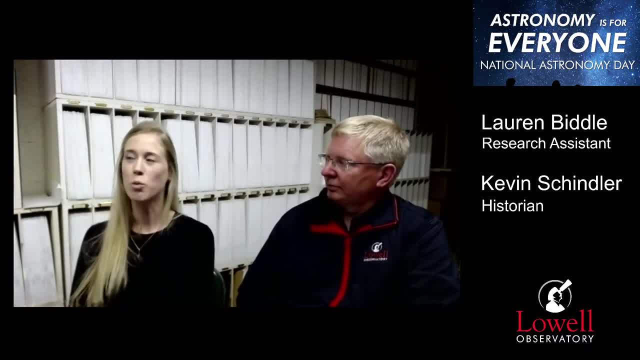 it is that i can go out and i can look up and say, right, this is where i am, this is where we are, and, um, that's something anyone can do. yeah, it's, it's available to anybody, you don't need any special equipment. um, you can look up, and and even if you can't look up, 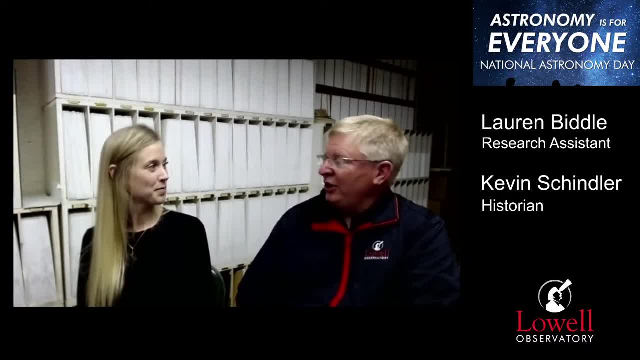 um, there are other ways of of enjoying the universe around us, um, and yet you're somebody who not only enjoys it, but are helping us understand this. so people that are watching down the road as they learn more about space is because you and your colleagues, and so it's. it's. 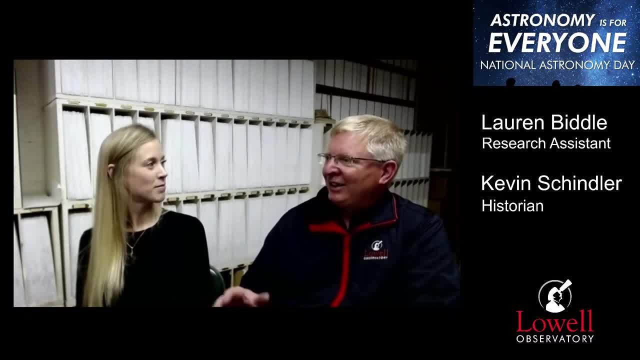 really enjoyable for us here at the observatory, you know, to have that mission of of sharing discovery and sharing the excitement of the universe um, and that means you going to science conferences and and um revealing your latest finds, or or this new method for detecting exoplanets. 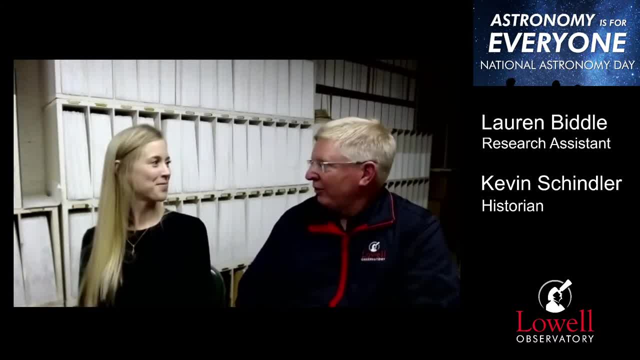 it's also you talking to. you've probably talked to some school groups or um. have you done any teaching as part of your undergraduate or graduate work? yeah, so i've done. um. i've been a teaching assistant early in my graduate years and that was so much fun. 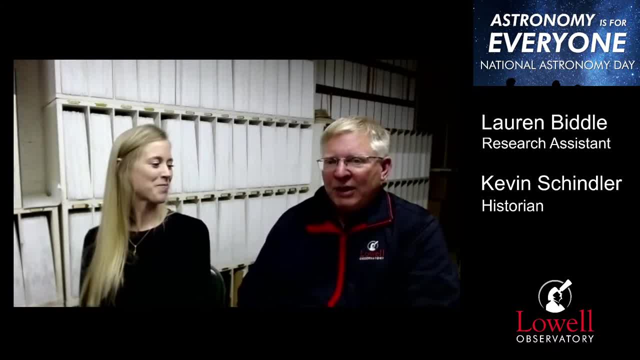 i loved it. and we have another question from david moore, um, about the, the james webb telescope and um. david asked if it ever launches um, and i think that's what a lot of us ask, but it seems like it's. it's really going to happen here, um with james webb um. would you use that in any in your studies? 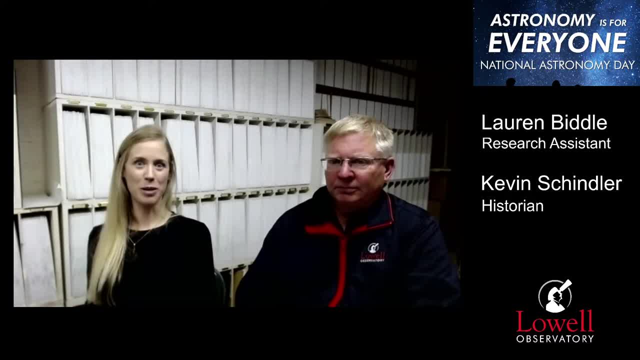 i absolutely could. um, so the james webb space telescope will probably initially be pretty, um, uh, subscribed, oversubscribed, so, like what we have to do is apply for time on these telescopes and then, um, there's only so much time and it really kind of makes you aware of, like human. 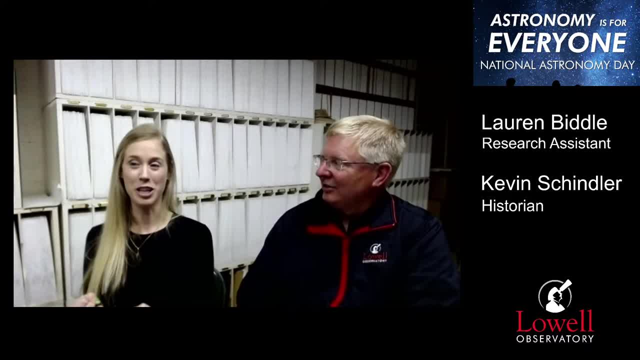 time scales too. you're like, oh, but i you know i only have this much time to do to answer these many questions, and so really, it just requires a lot of persistence and then you will get some space. you will, you will get time, and so when we do, i would really like to 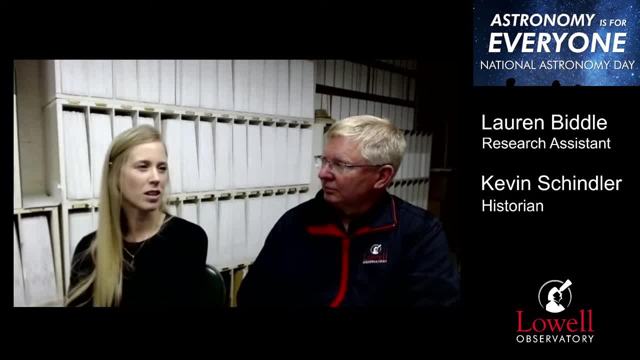 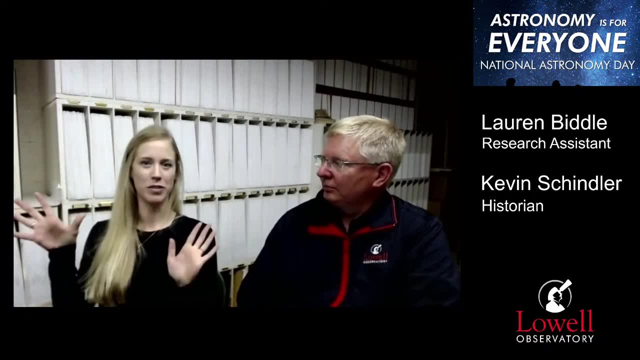 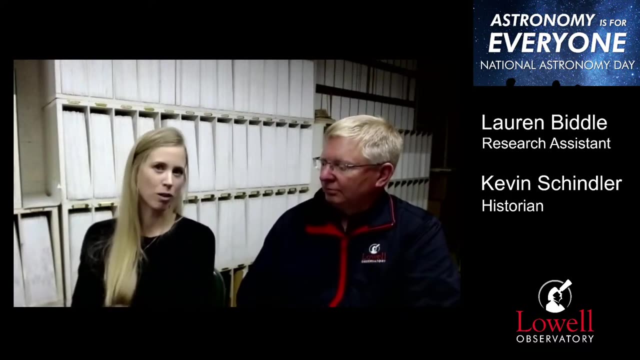 look at um these discs even more. i guess, like that's like it, just, it's just. you have more photons with that aperture of telescope and it's in space, so, um, it's going to be great for imaging, especially like direct imaging of planets. i think would be really cool. i don't have. 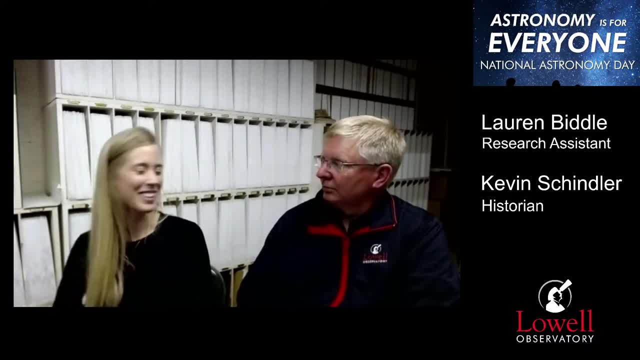 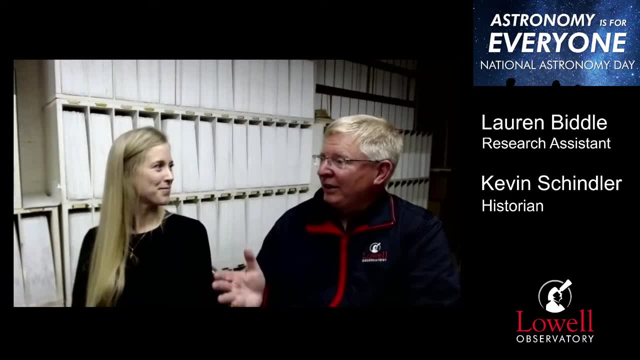 experience in that, but i mean, i'm young, maybe maybe i will. um, yeah, that'd be great. and and you bring up something that's really cool about the james webb space telescope. that's really important with astronomy: is you know, as an astronomer, to use a telescope somewhere? 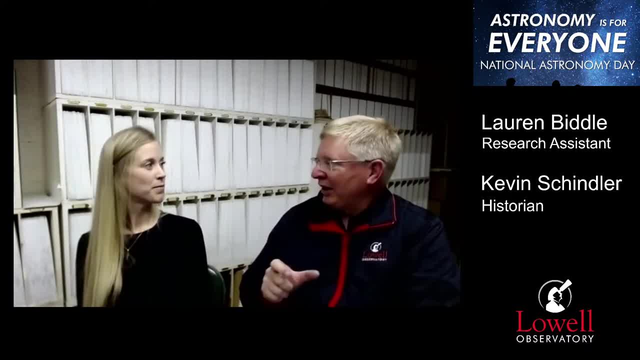 you're competing with other people and there's only so much time on a telescope to look at the sky, and that's one of the benefits here at the observatory. um, while some of our astronomers, like you said, use different telescopes around the world, we also own our own suite, including the 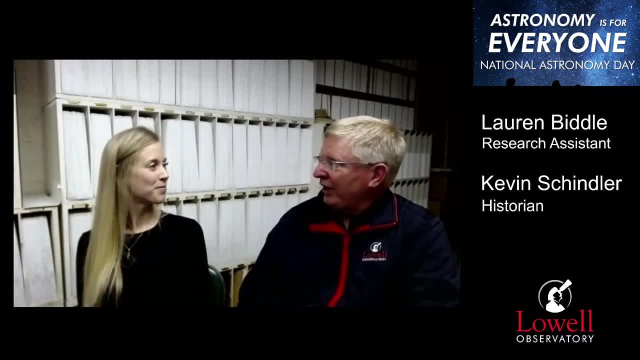 little discovery telescope, and so that gives us the flexibility to you know, especially if there's something really cool happening we can. we can use the telescope to look at the sky, and so that's one of the benefits here at the observatory. um, while some of our astronomers, like you said, 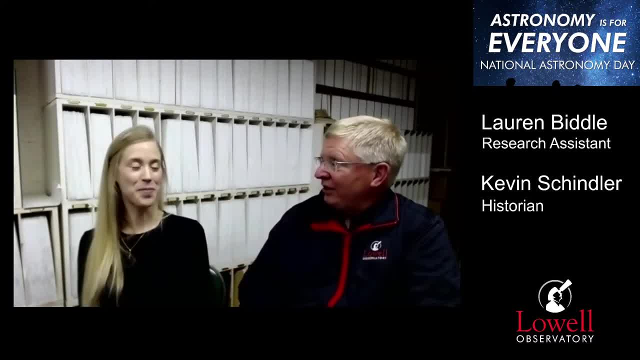 reposition and look at it pretty quickly where other places the telescope's already subscribed, and so that's the benefit we have here: the flexibility of having your own telescopes. um, have you used the ldt? i have, yes, and what? what's instruments and what were you doing with? 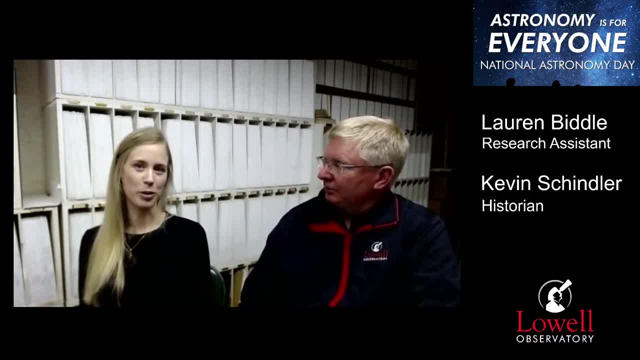 that i used um lmi, which is an imager. we were actually taking measurements of planet transits. so that's like i said previously: when the planet passes in front of the stars and then we're looking at the star, the brightness of the system will get dimmer while the planet is in front and 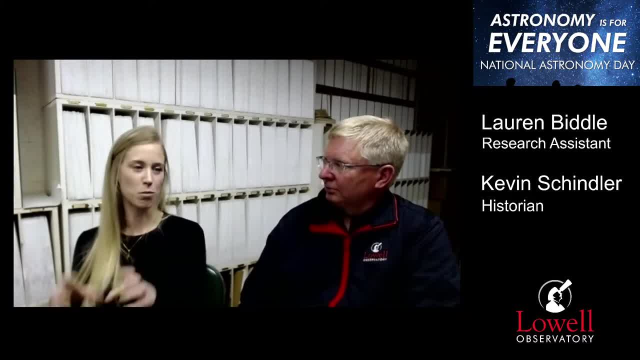 so we were uh looking at those transits in multiple different wavelengths, because the atmosphere of a planet will uh, depending on what it's made of, it might absorb in one wavelength of light and not in another, and so if we see that that dip in brightness is different for one wavelength, 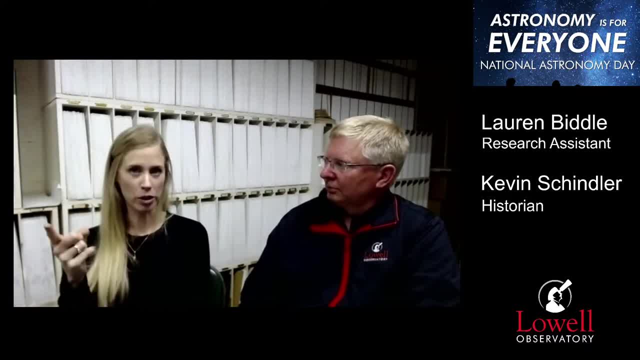 versus another. we can say, oh, we're going to have a different wavelength and we're going to have a. well, it might have this molecule in the atmosphere, and so that's one type of science that we've done with the ldt um. we've also taken spectra using express, which is a really cool instrument. 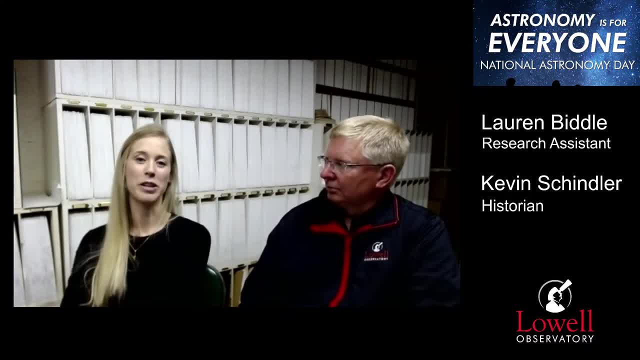 to get really high precision radial velocities, and so that's um that that is. this is what it's used for often. that's when the star will wobble under the gravitational influence of a planet that would be orbiting around it, and that planet doesn't have to transit. 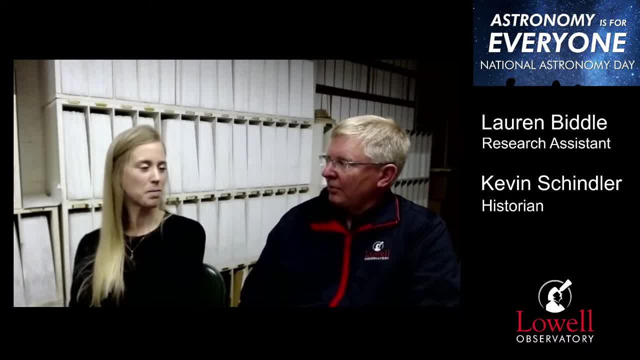 like the science i was talking about and express is a good example of, again, the partnerships in astronomy, um, both among people and institutions, because it expresses the spectrograph that was built by yale um, and there are partners on this, so maybe you can talk about express the larger. 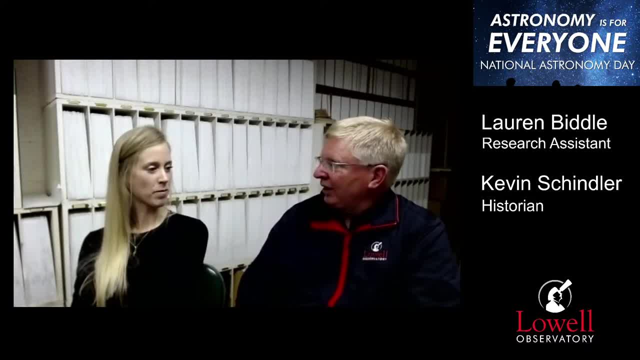 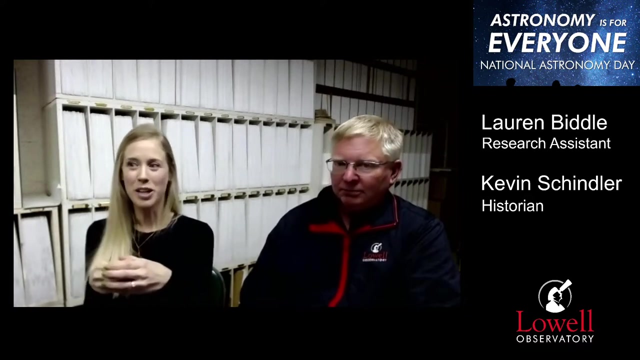 um picture of of why it was built and what, what they're looking for with it. i mean, well, you, but others like, like um, deborah fisher, and and our team with joe long, when you mentioned yeah, so, uh, express, uh the. the primary goal is to be able to detect those, uh, those that wobble. 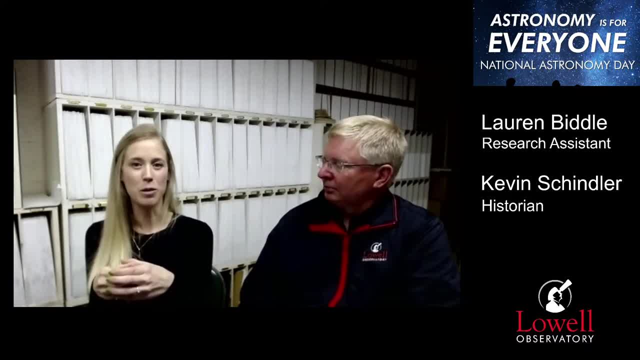 down to, i think it's like a meter 10, a centimeter per second, uh change in the stars wobble because, uh, the reason we want to do that is because we want to be able to detect those, uh, those wobble, and we want to detect it. so, uh, precisely a doubt, like all the very faint wobble, is because 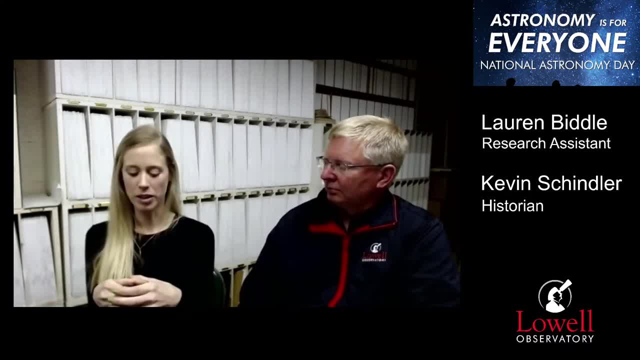 the, the mass of the orbiting planet, uh, really dominates how much it's going to wobble, and so if we're going to look for earth-like planets, they're not going to be as massive as, say, like a jupiter. and so we find a lot of jupiters because it's so easy to detect and we want to. 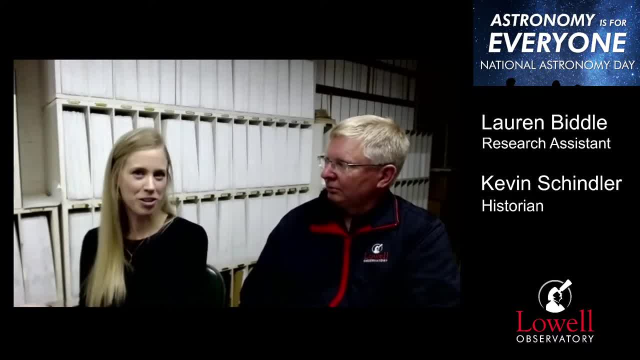 detect that wobble, but we haven't found a lot of earths that way, and so this instrument is designed to say, okay, how, how, how small of a change in that star's wobble can we detect? but can we optimize that? because the more we can do that, the the more likely we are that we can detect a planet like. 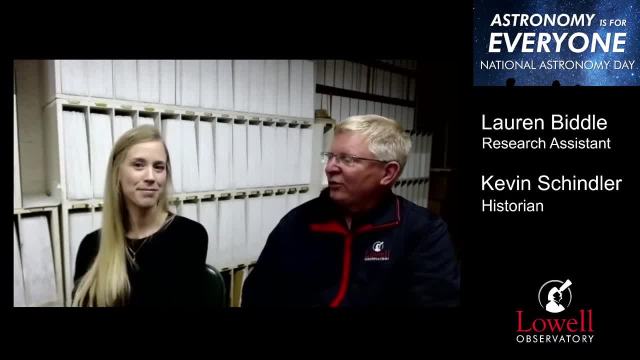 earth around a sun-like star. so when this was being built over the last few years, you must have been giddy: come on, let's hurry up, get this thing done. yeah, absolutely. i mean, it really revolutionizes how we're searching and what we expect to find and and you're on the cutting edge of it, so that must be just really. 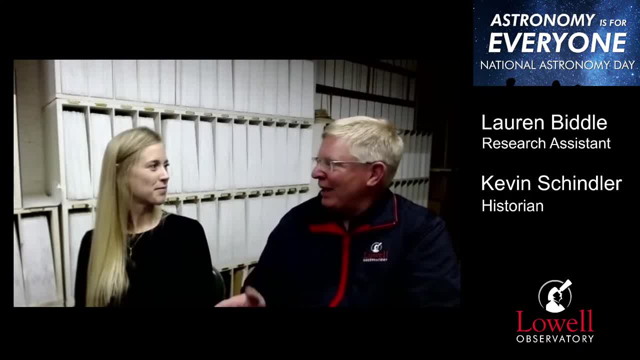 neat, um, to be at a place where that's all happening and you get to use it too, and that's just really neat. yeah, and you can use it for science, um, beyond just um, radial velocity, observations of wobbling stars. i've also used it to, uh. 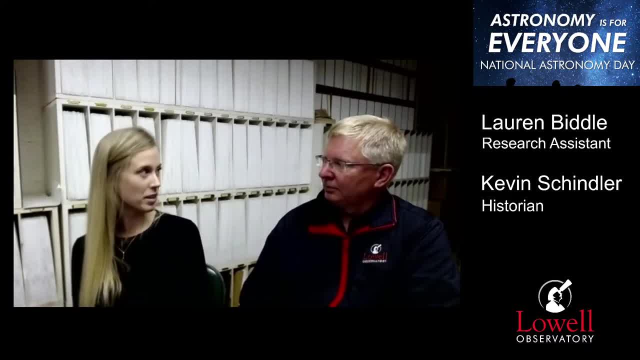 test it, and i've also used it to test it, and i've also used it to test it, and i've also used it to test our ability to detect prominences on young stars. so the sun also has prominences. if you, uh, came up to low observatory during the day, there might be a telescope out that's looking. 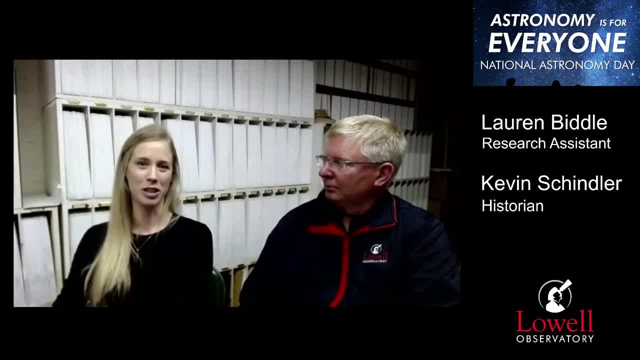 at the sun. it has to have a filter on it, of course, because you don't ever want to look at the sun, with or without a telescope. but, um, you will see these like uh, uh, they kind of look like hairs on our sun that are coming out of the side and those are prominences and it's just like a lot of hot gas. 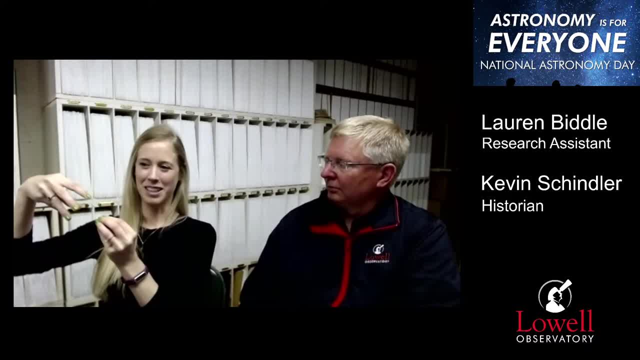 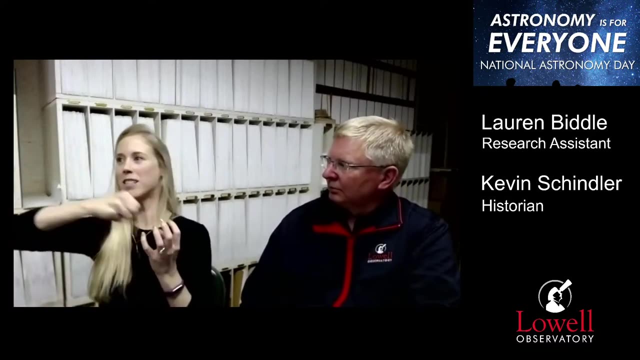 that's and that's being um, uh shot out in the on the magnetic field and it just kind of hangs there, and so these also exist on young stars, but they're way bigger. like these prominences will extend out several times, uh, like the radius of the star, i think- and they'll hold. 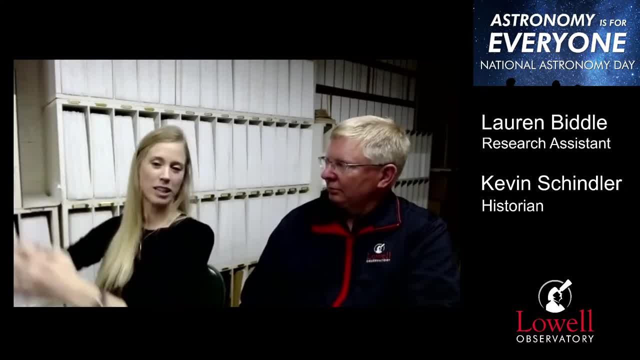 uh colder gas and they'll hold uh colder gas and they'll hold uh colder gas and they'll hold out on the edge, and so we can also look for that signature um in spectra, and that's what i used express for also. yeah, so a lot of different things you can do with it. that looks like we have a couple. 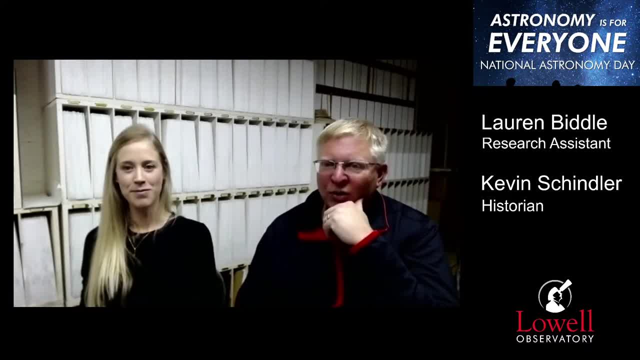 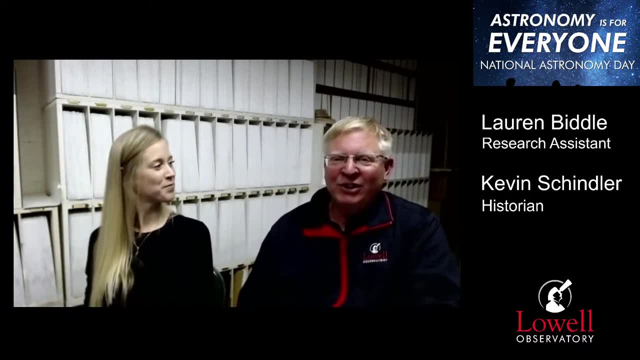 more questions here. um one, david moore. oh, david is mentioning about charles capon. um a little observatory, um chick capon, he was, uh, i, i think he was a student of clive tombaugh's, in fact, at new mexico state university. um, and he was a student of clive tombaugh's and he was a student of. 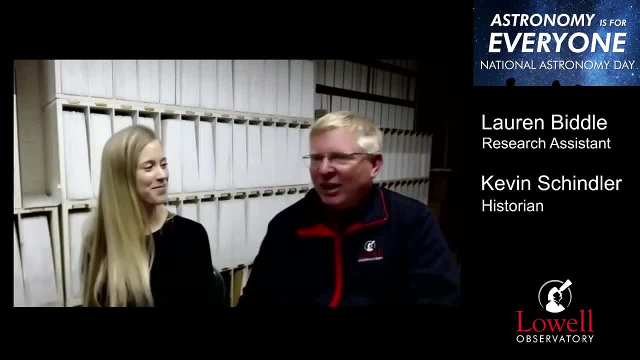 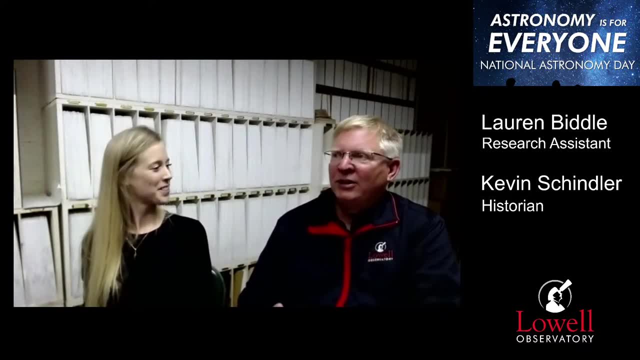 we're, you know, the top several rows here, or clive tombaugh's handiwork, um, but chick capon was here at the observatory in the, i think, the 1970s and we have this classic picture of him that well, if i go. 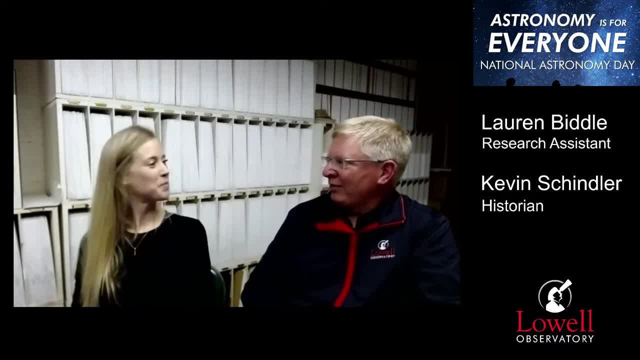 back a little bit. the iconic image of lowell observatory is percival sitting at the top. yes, um, chick capon- i never met him, i haven't met him, but um, he used to do tours here in addition to research and he would dress up as percival lowell and we have a picture of him sitting on the chair. 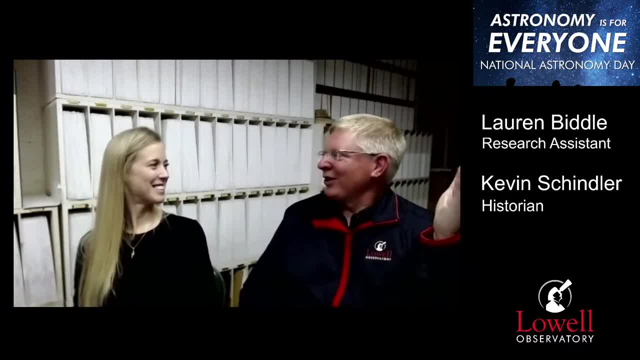 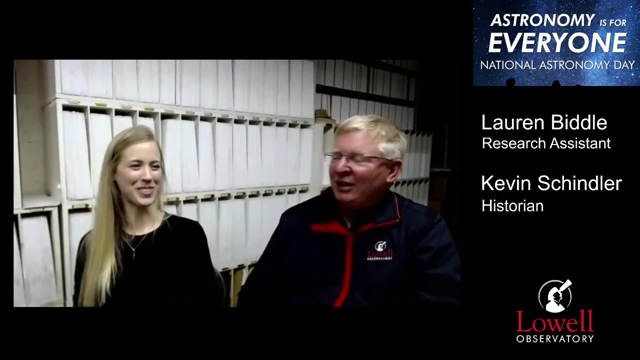 at the same angle with a cap turned backwards. i'm just like percival lowell did so by. by my understanding, he was quite quite the educator and just like you know what you're showing, is here somebody interested in doing the science but also sharing your excitement with people, because our just like that, our founder. 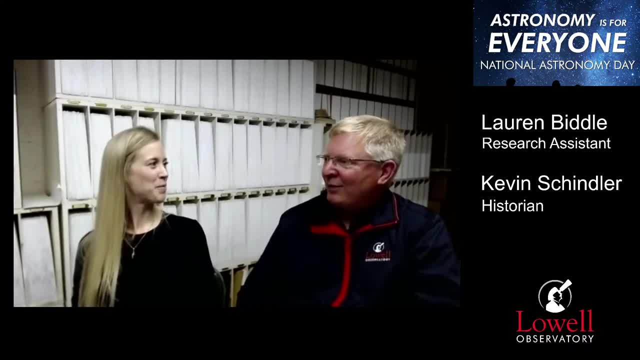 percival lowell essentially said: we want to do science, but what's the point if you don't share it and make it accessible to people? and that's that's what we do here and um, it's, it's a, it's a great thing. you know, we're actually a company from the university of california, so it's. 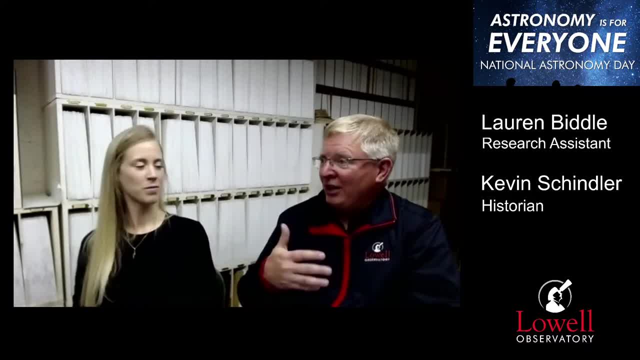 already an organization that has been practicing with elon musk for thousands of years now and, of course, my first smart phone call to me was about to ask you about taking a photo for a photo. um, so we're looking at, maybe in February- what's the date of the first photo that you're taking? 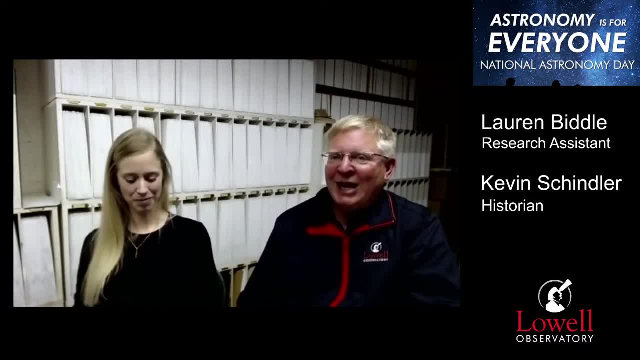 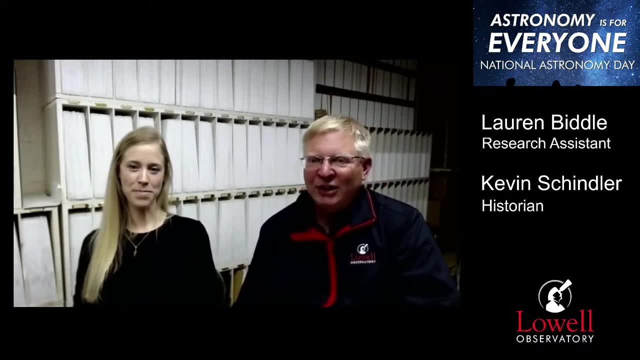 you know the date of the first photo of the laviata: the following day, so we're hoping to run that out the next day, and that's what we're doing, and we do have a lot of work to do, and we're. And we have a question from Christy Engel. 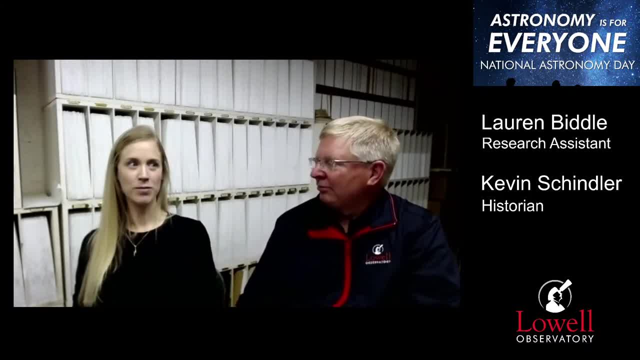 Have you published your findings And, if so, where can people find those? I have published my findings And until recently there hasn't been as much discussion about how to make published works available to anybody. But that is changing. Recently the AAS has announced that's the American Astronomical Society. 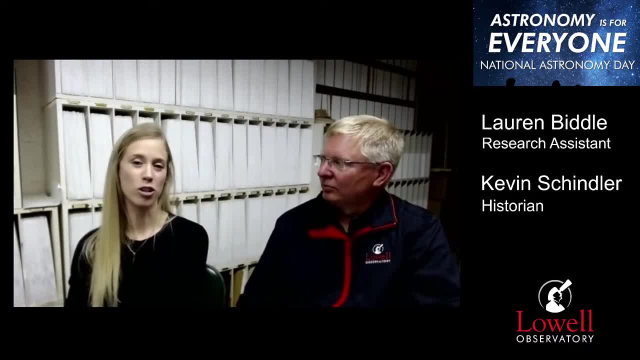 They have announced that their journals will become open source soon, meaning that anyone can read publications in their journals. Until then, I'm not exactly sure the timeline in which that will go through, But until then, a lot of researchers will post their works to an online site called Archive, which is also open source. 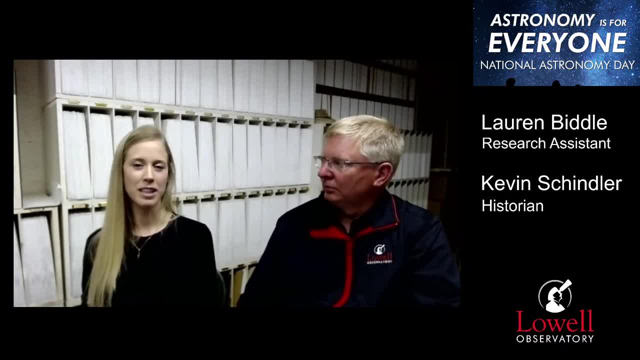 And it's AAS A-R-X-I-V And you can. it's not just astronomy. There's actually a lot of really cool science that's published there that anyone can access, And I would say: go there for now at least, until the AAS journals become open source. 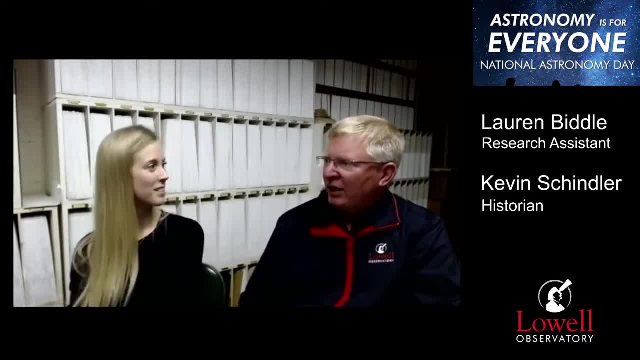 And that, really, that's really changing everything. I mean, well, just like everything used to be printed, Now you know, more and more is digital. Eventually, all research is going to be printed. It's going to be digital. 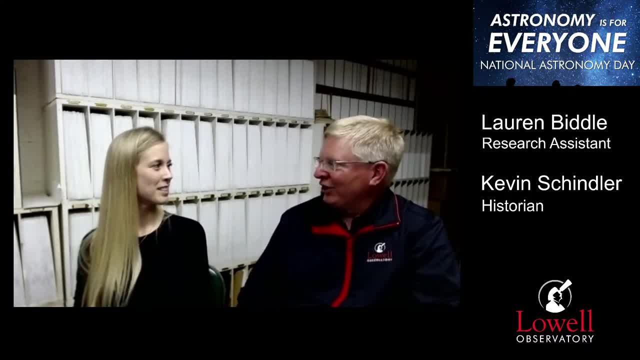 You know libraries are one of the things that aren't. they're not growing that much now because you know journals are going to digital. It just changes how we do a lot of things, But it's nice to be able to have that accessible. 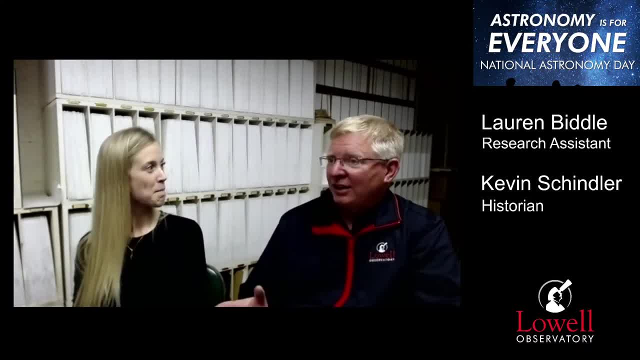 Yes, I know, for my part, sometimes you know writing about a discovery and wanting to see the paper but you can see the abstract but then you have to subscribe But to be able to see the entire paper- And you know a lot of science papers- the typical person not doing astronomy may not last more than a couple sentences to where you know they find something a little, you know, maybe more interesting with all the numbers and stuff. 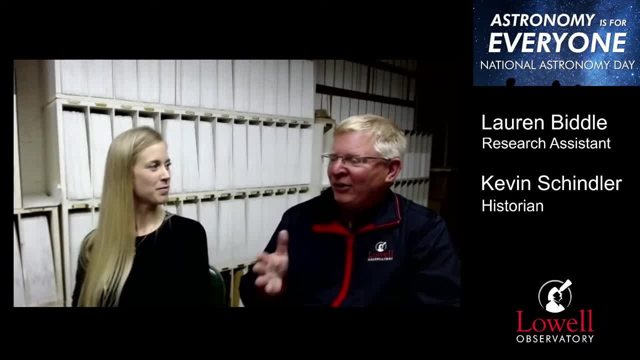 But on the other hand, I don't know every paper that I've seen. you get something out of it, Even if you don't have a background. you get the gist, You know. so I summarized what was the important finding here. 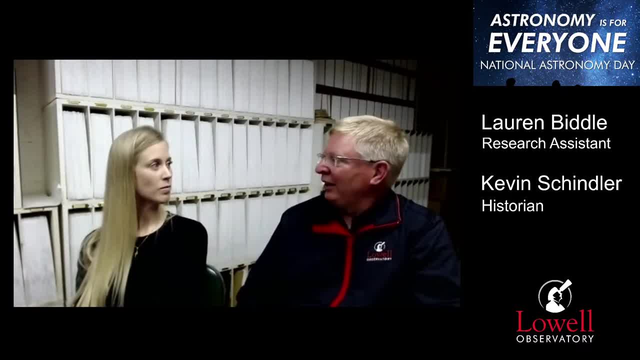 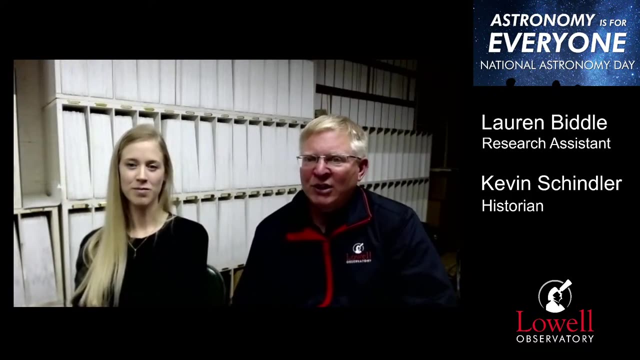 And even if you don't read everything, you know just scanning And you know the results can be really informative and exciting to see just the diversity of what's happening. I'm going to say we've got another question here, Again from David: is there anything amateur astronomers can do to assist your studies, assuming proper telescope size? 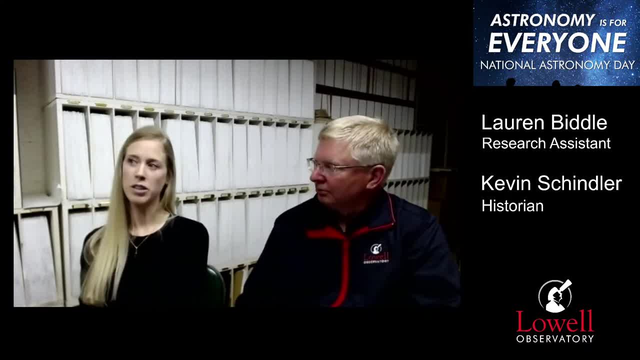 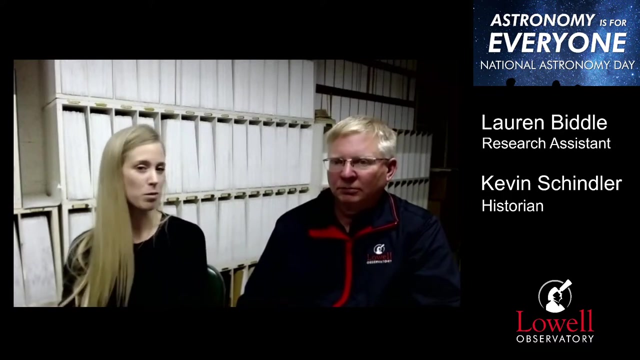 Oh, I do know that some amateur astronomers have collaborated With professional astronomers. There is actually one that does that is in communication with someone in my group, And so it is possible. It just takes some reaching out. But also anyone can can become involved in astronomy research with citizen science projects. 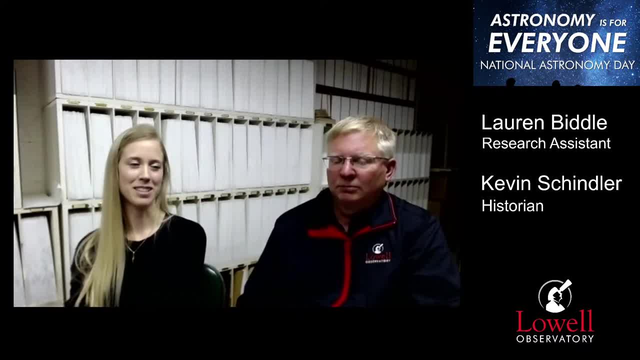 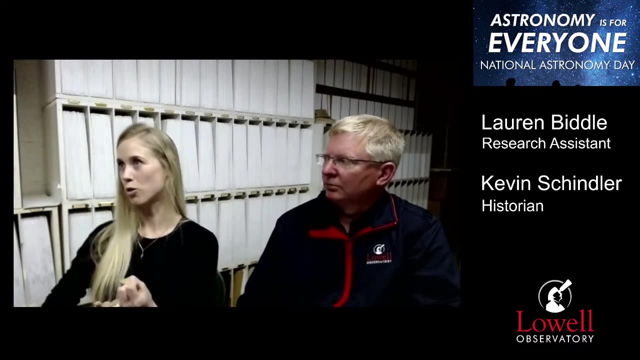 Those exist online And like. there's one called Galaxy Zoo Where anyone- Anyone- can go on and help classify galaxies. There's also, like, a lot of classifications that you can do for, like solar data, Like what, what type of spot is this? and like: where does that fit into the context of solar physics? 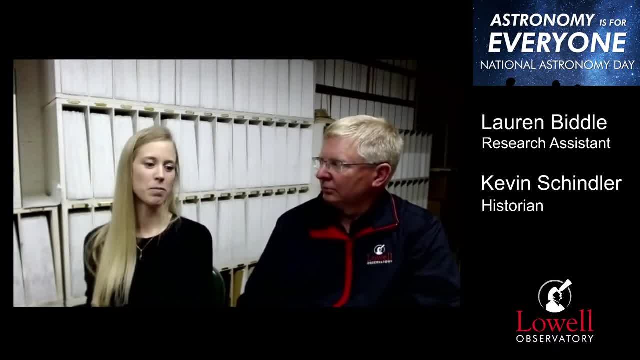 And it's not uncommon actually, for every once in a while someone will come across a citizen will come across something really interesting. The end That will be flagged up To the people in charge of the citizen science project- not citizen- could even become a co-author. 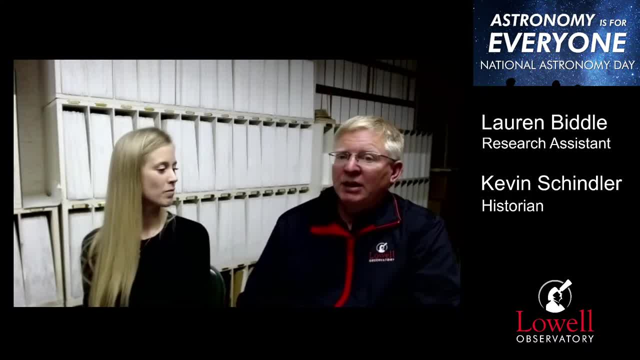 It's, it's not unheard of at least, And we've certainly had some some amateur astronomers helping with research. Gerard Benville had one of our astronomers here. I think he still has some some amateur astronomers he works with And for a time we've had- we had a program at one point. 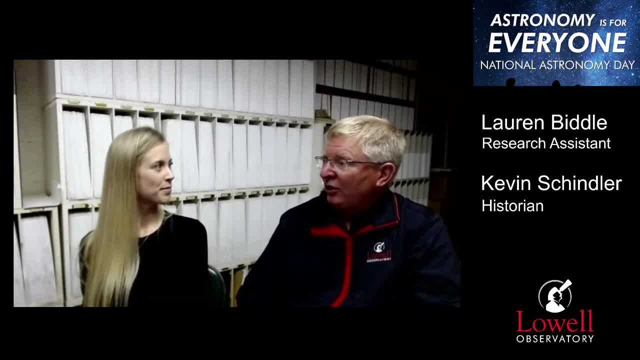 And so you know a lot of amateurs is neat When you go to a like a major Star party. there are some majorly telescopes that the amateurs have bought and and you know it's amazing, You don't always need the Hubble Space Telescope or the James Webb soon to make so many fundamental discoveries. 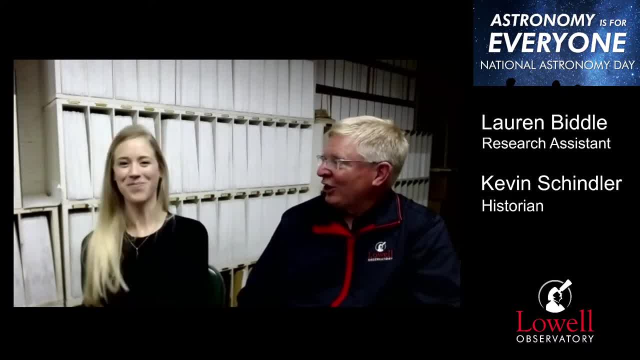 I'm like. I'm Georgie Mandashev, who was just in here a little bit ago. He was involved with the trace program, looking for planets and using- I think it was- a four inch diameter telescope. They discovered one of the largest. 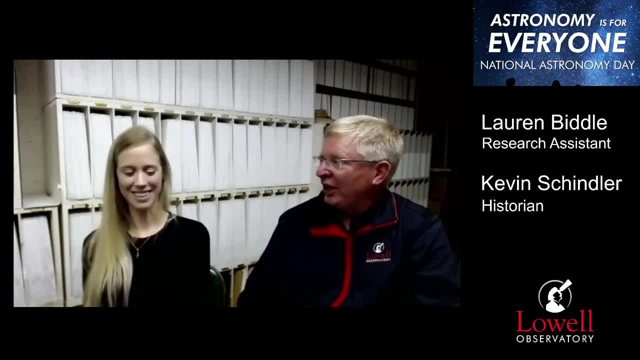 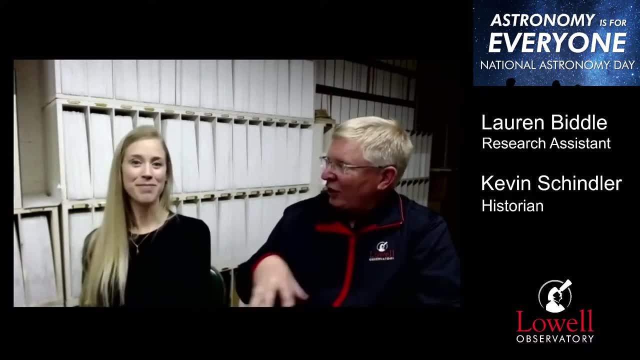 If not the largest known planet on record. as of right now it will change, But but there's, it's just. it's. it's the equipment, it's the people, the techniques. There's a lot of different things that go into doing research or even just looking at the sky. 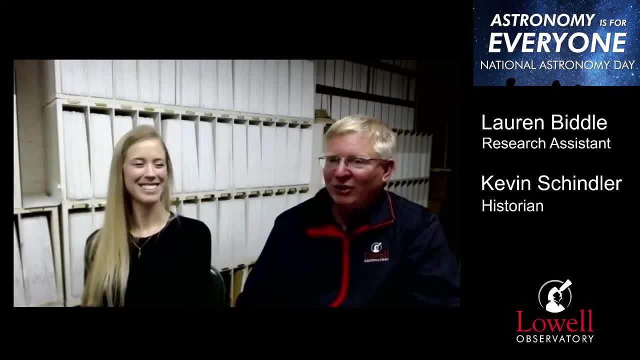 And so you don't have to have the Cadillac necessarily to do a lot of that. So we have another question here. If you know politics, political borders, money, resources, if none of that was an issue, What would be like the coolest, the most important instrument or equipment to do astronomy? 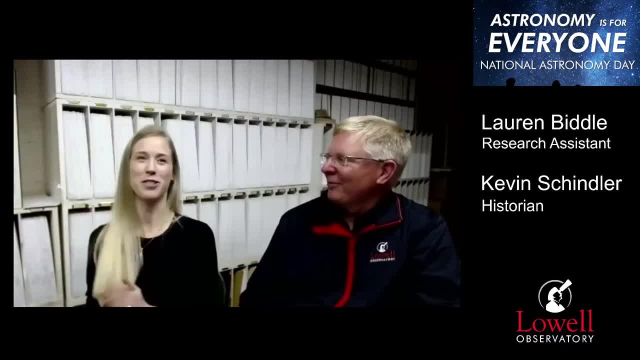 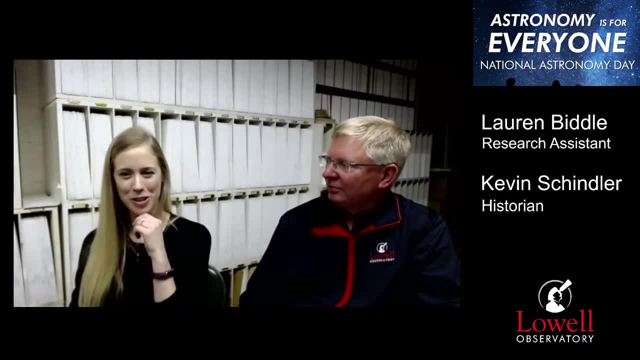 Money is no object. Oh, that would be so cool. OK, so I'm not sure if my, if my, if I'm answering the question necessarily because it made me think of what's my dream telescope. So I'll address the question first and then I'll tell you what my dream telescope is. 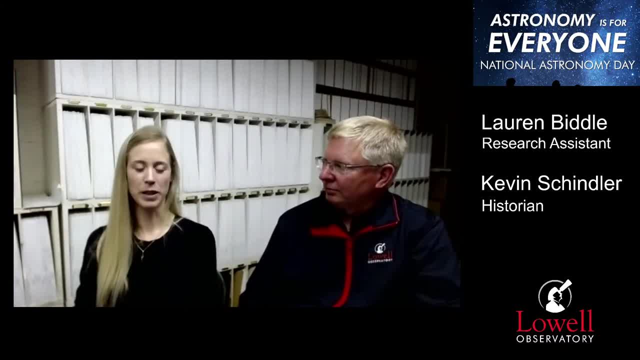 So I think the field of astronomy, Like as a whole, would really I mentioned, would really benefit from having more facilities, really observational facilities. I was saying earlier that we have to apply for time To just to do our science on many telescopes and we've had to compete with other astronomers for that time. 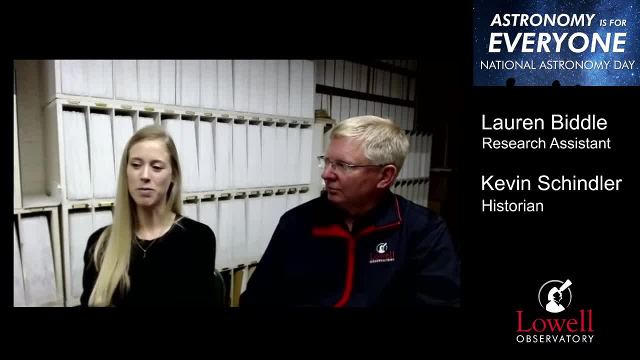 And so I think that that that wouldn't be as much of an issue if we just had more large scale next generation observing facilities. and So what's your, what's your dream telescope? So my dream telescope is A very large interferometer that exists in space, and so an interferometer. 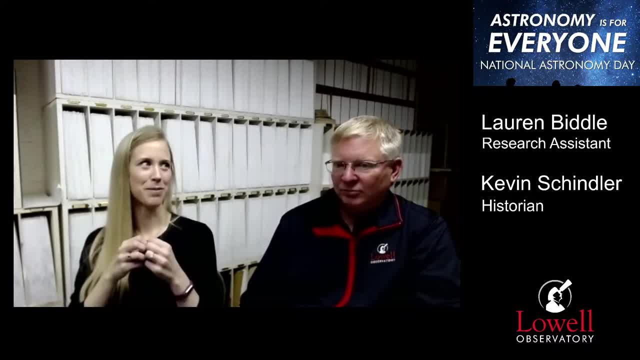 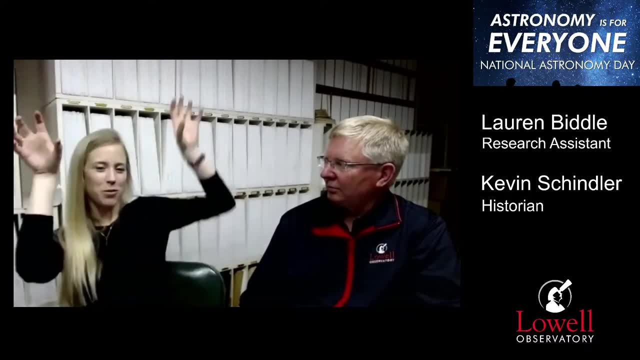 Is a telescope. well, it's like a, it counts as it's like one telescope, but really there are multiple telescopes really far apart from each other, and then they can combine to form an image and what it allows for is extremely high resolution images. so, when we doesn't matter right now the telescopes that we have, no matter what the 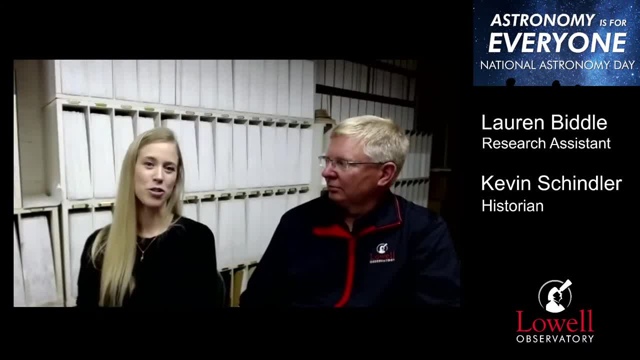 So when we doesn't matter right now, the telescopes that we have, no matter what the The stars Actually looks like to us, it's still going to look like points source, but if we have a large enough interferometer with a long enough base line. so that's the distance between the 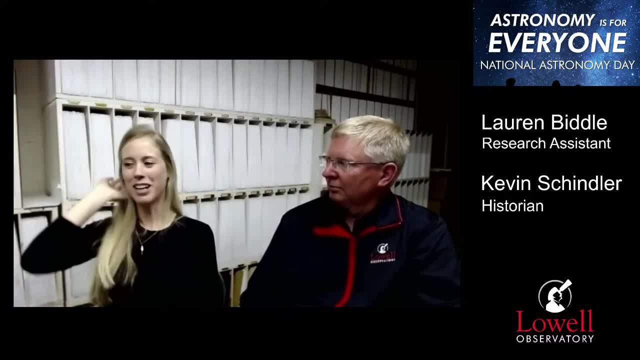 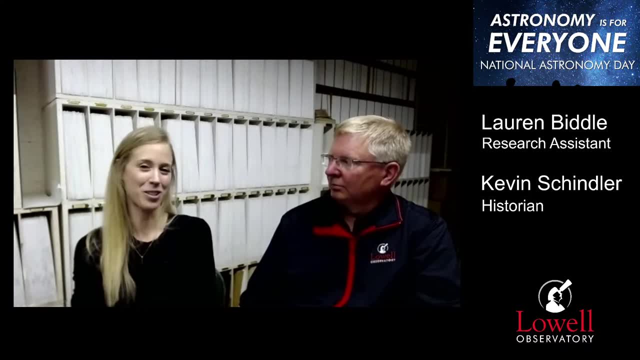 Individual telescopes that would make them combined to form the image. I think that we would be able to actually image stars And their services and and start forming systems like micro research with very high resolution, And that would be that would be so revolutionary. That would answer so many questions that we have. 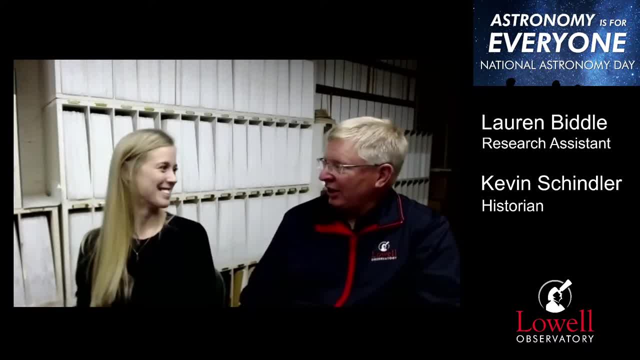 Yes, And maybe you can talk a little bit about Lowell's interferometer and what's being done with that, The one that's not in space but is here in Flagstaff. I know you don't use that or you've never done any research with that right. 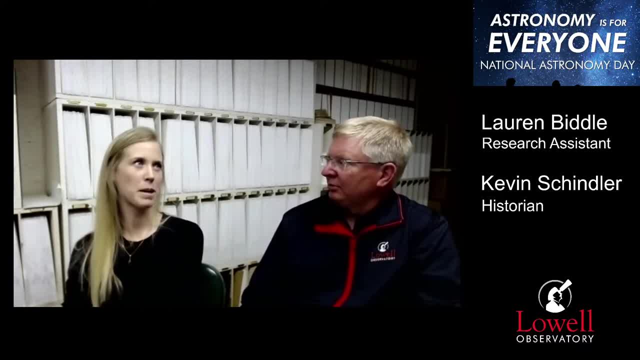 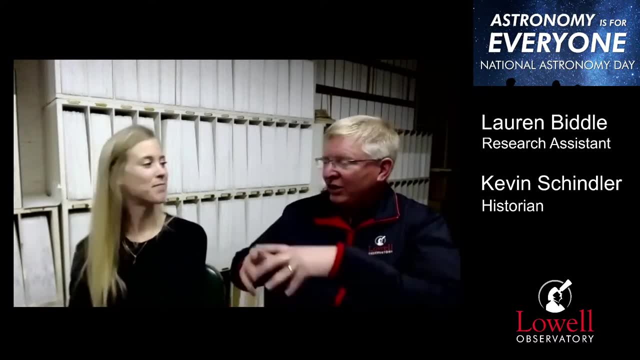 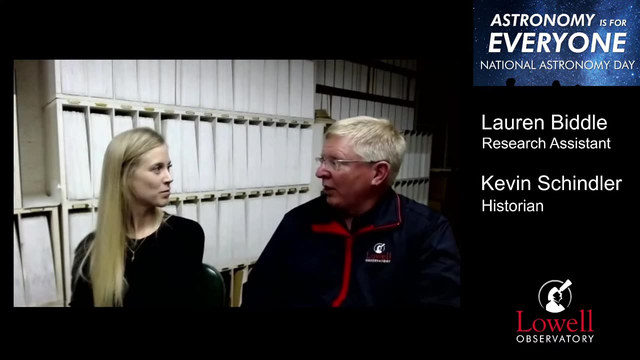 I have not. I'm actually not as not as familiar with that. Well, it's like you were describing an optical interferometer with dishes spread out over several hundred yards, And we'll be expanding that to where it will be the largest one in the world. 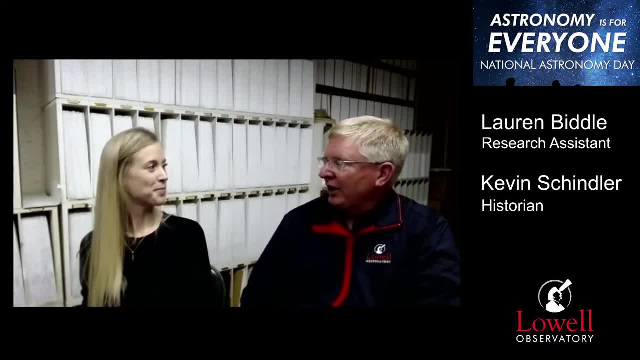 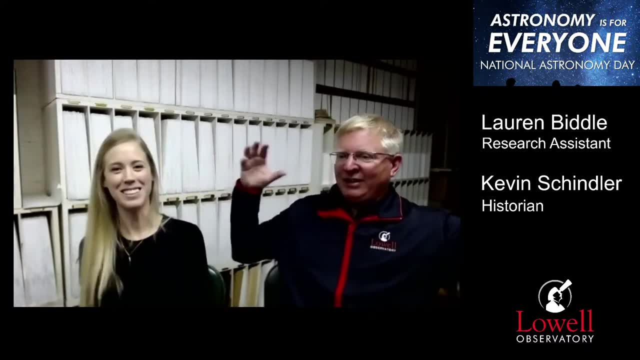 I mean Gerard Van Bell is heading that project where it allows you, like you were saying the resolution, You have to look at bright objects because it's not like you have one big mirror. It's always a mirror. It's a bunch of smaller ones but they're spread out so you can see an object from a lot of different angles to get a good resolution. 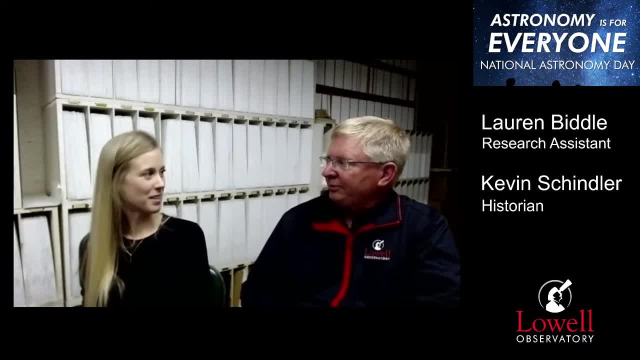 But they have to be pretty bright to be able to see it. Yeah, And I do know that it is more difficult to do in the optical. So, like what I mean by the optical or visible wavelengths- light that our eyes can see, And I think that's, those are the wavelengths that that interferometer combines. 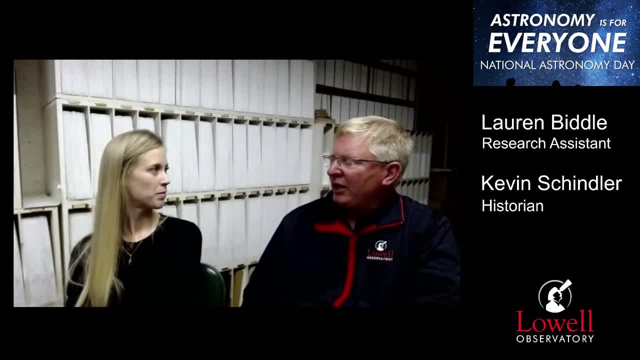 Yeah, we, that's. it's called the Navy Precision Optical Interferometer. So we work with the Naval Observatory and the Office of Naval Research. It's a big partnership And it's a. it's a magnificent instrument When you see it how it works and everything using vacuum tubes to send light photons back and forth. 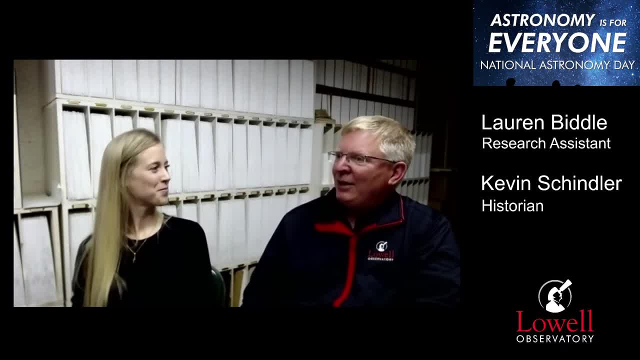 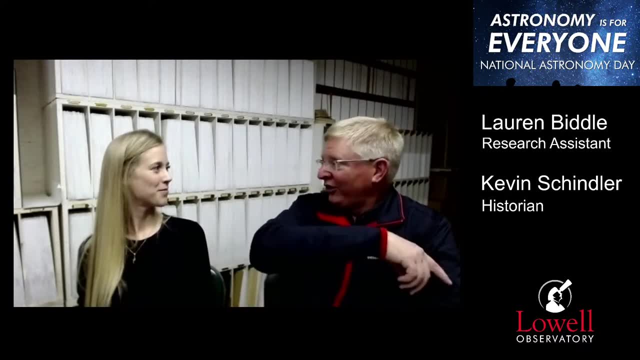 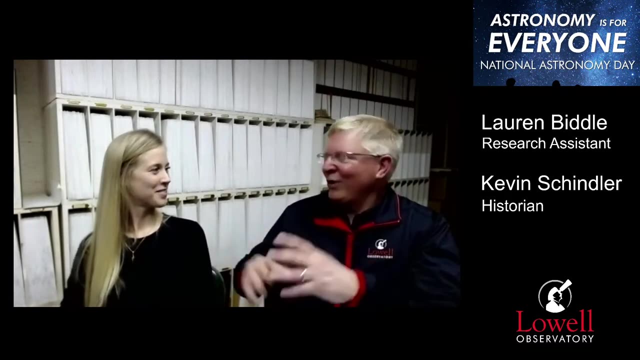 It's really. it's really a high tech thing, But it's neat because it's located, you know, out at Anderson Mesa, our dark sky site across from Lake Mary, And the Arizona Trail is nearby, So you can walk by and it's fenced off, but you can still look and see this really weird array. And this Y-shaped pattern is. it's really neat to see, Kind of like the LDT, the Low Discovery Telescope. You drive down Lake Mary Road and suddenly there's this big like flying saucer looking thing in the middle of the woods. 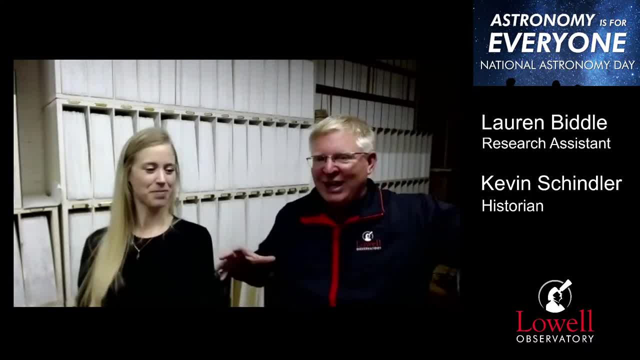 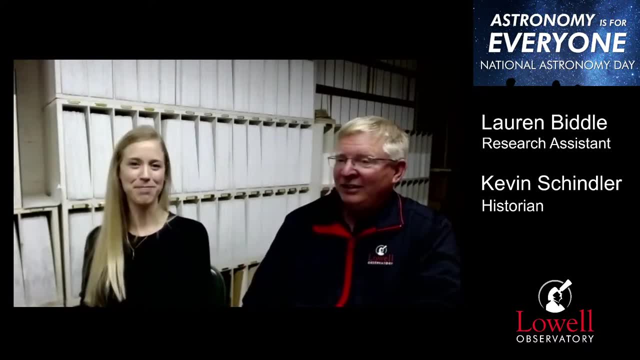 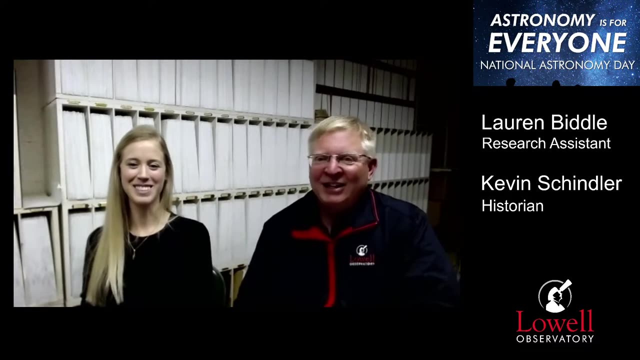 And it's this: this 14 foot diameter, 4.3 meter telescope And there's dome that are out there. And it's out there because it's dark And the seeing conditions are good. So let's see The statement. how you answered, it was just that they're looking for kind of a- you know, reach for the stars side of if you could have everything. 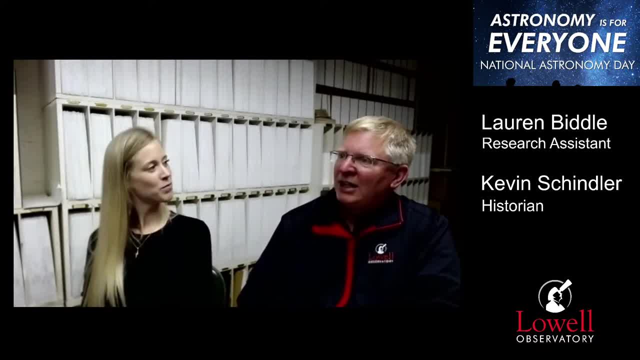 Now, now it does bring bring up something I think is interesting. You know, we have, we have people that are going back into space, And we've been, we've had, Yeah, Astronauts going into space. but commercialization is redefining what it means to go to space. 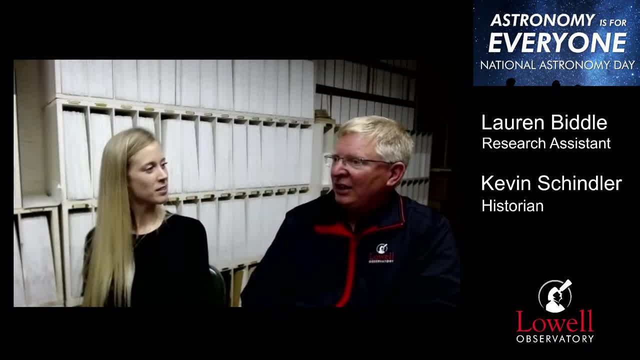 And it'll be interesting to see what impact that has on science, as private companies work with NASA to go to the moon and elsewhere. But you know that costs money. The privatization is one thing, but for a long time there's been an argument. 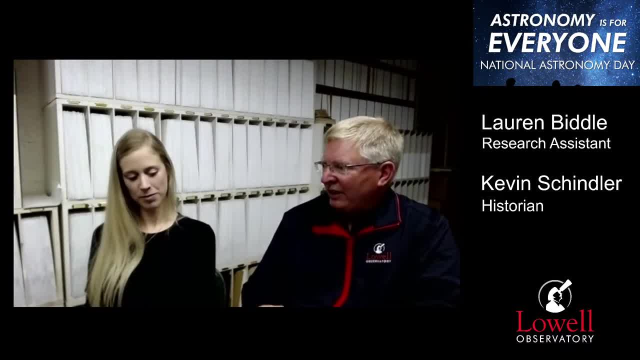 You know, if there's, if there's, if NASA, for instance, has only so much money, Is it better to to send People into space, Or for a lot less money, and you can do a lot more in some ways. 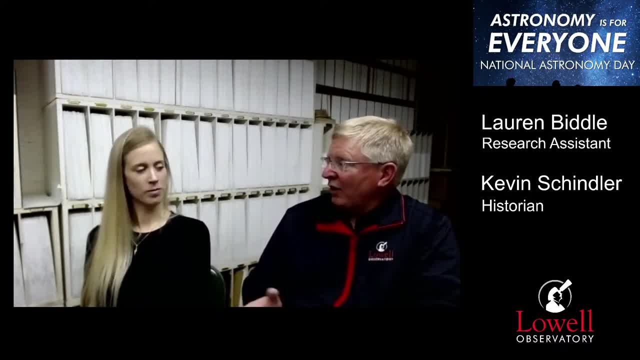 To send unmanned or uncrafted, uncrewed craft into space. Or don't send any craft and just use the telescope we have here and bolster them. I mean, what do you think about all those You know is there? is there a better solution or how, how we should spend that kind of money? Hmm, I think Yes to all that. I think that any way that we can do it, we should, And how? whether it's privatized or not, I'm optimistic for humanity's progress in exploring the cosmos in a physical sense. 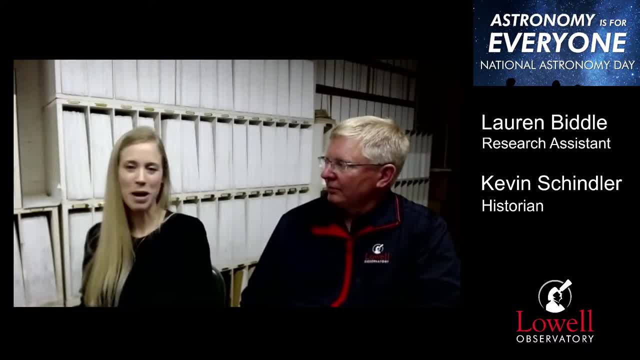 And so I am. no matter how it is done, I am all for it. Yeah, And you know there's something? because we're as human beings, we're inquisitive, just like you've been all your life Asking questions. And To be able to send our species to another world. I mean, you, could, you, could you. you know the the technology we got out of going to the moon, all the spin offs and you know, from medicine to microwaves, to our watches and cameras. 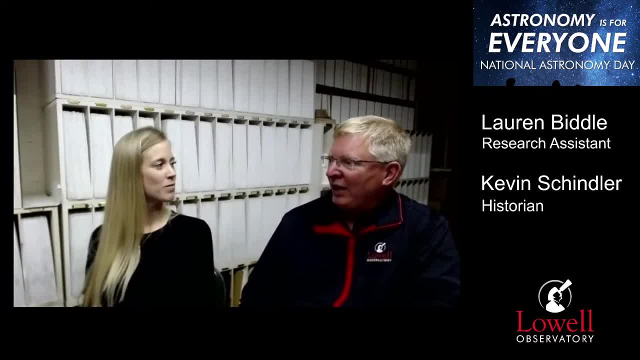 The way we live today is a product of the space race. But but even without that, the you know, sending a human, our species, somewhere And describing what the universe looks like. I mean there's, there's that human part of it. 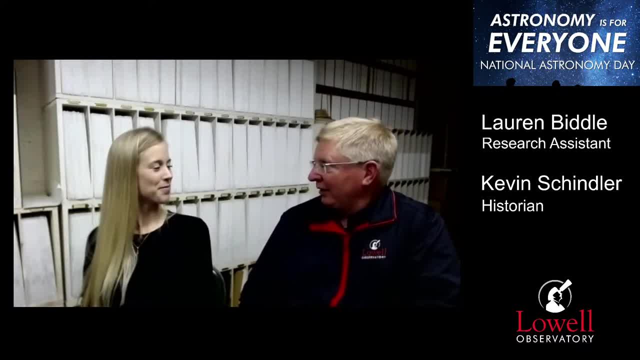 And even though you're not going into space, at least yet that we know of, I mean your ability to share the research, And that's that's what inspires people, That's what makes it. You can look at numbers And you can look at results. 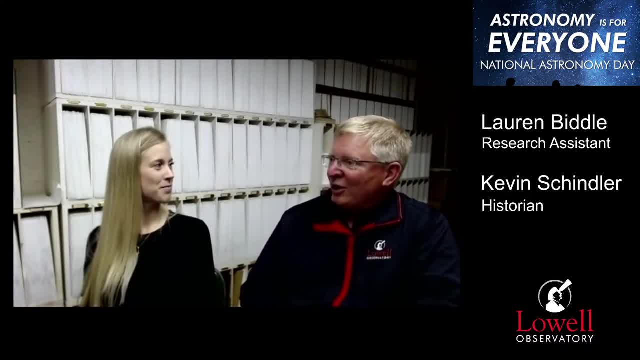 But when you hear how people did it, Are you hear about Like the old days of like like tomba, Sitting in the in the cold telescope dome- It can be 10 degrees Inside there- Looking through this eyepiece for an hour? 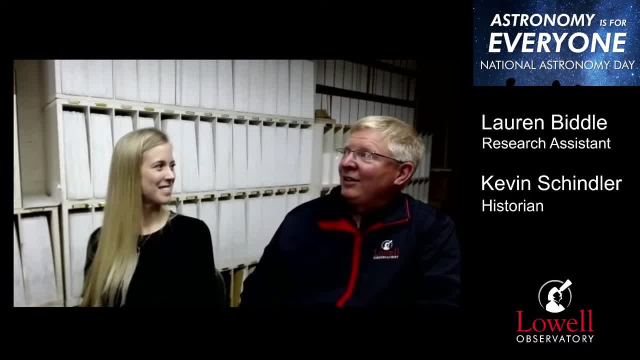 Trying not to fall asleep And then Developing those images. Looking through this machine called a blink imperative race. He spent A total of 7,000 hours of his life Looking through this eyepiece At millions of dots. That's hard to grasp. but but when you? 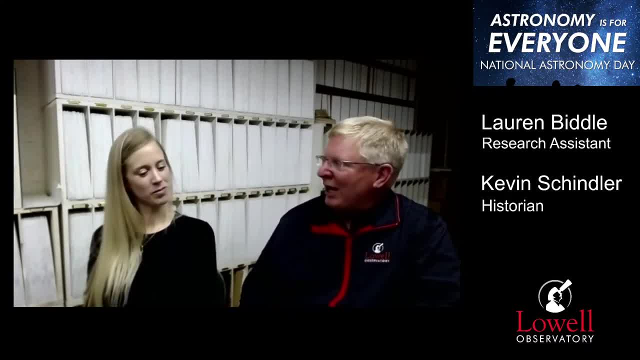 When you hear somebody describing it what it takes to do science, it really makes it A lot more fun, I think. And so there's that value of the human, the human experience also, So like in, in, in your experience. 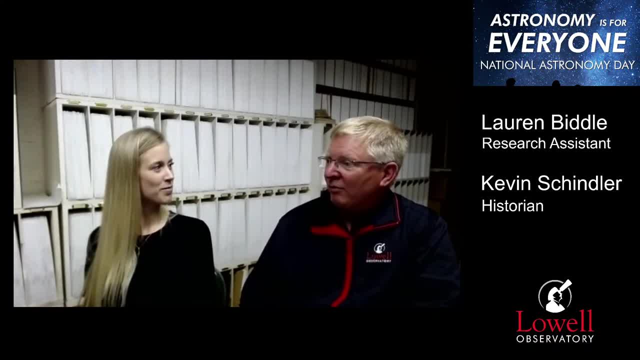 What's been your Like coolest astronomy moment? I mean is: is it You know that? Like the results of a paper or Looking through a telescope When you were in space? I mean, is it You know that? 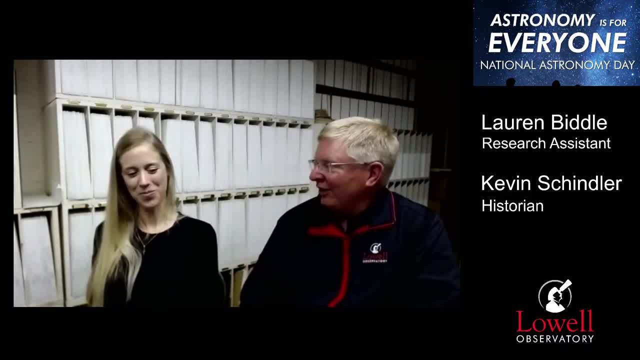 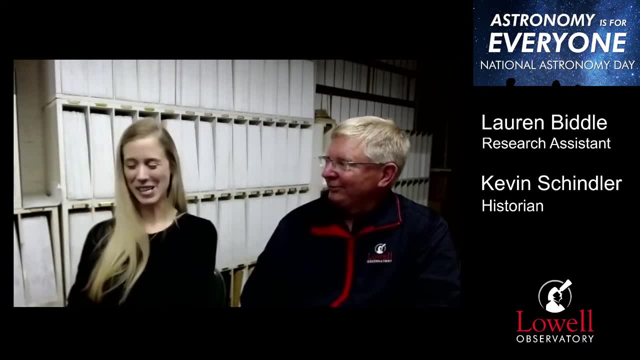 Like the results of a paper Or A telescope when you were eight or you know what. Is there one thing that just really jumps out is The coolest thing? Yeah, So it's going to be a tie Between the the moment where I actually was. 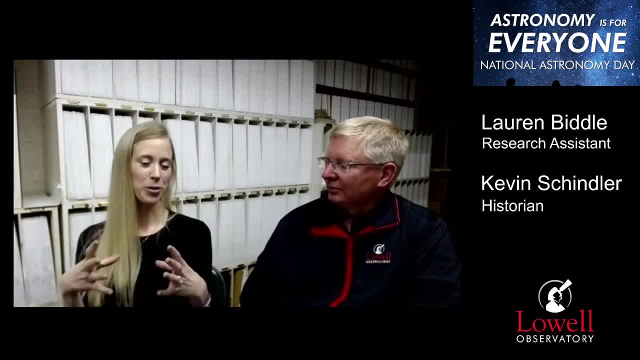 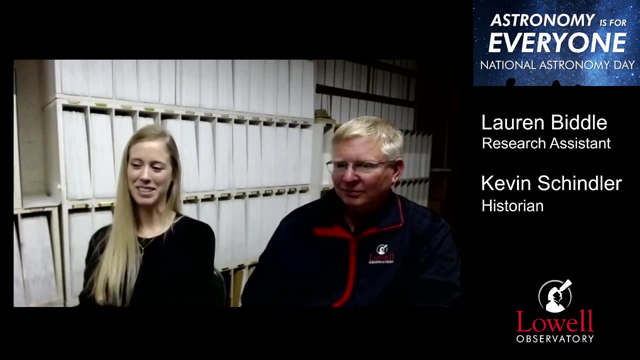 In Florida with my Papa Looking through the first telescope that I've ever had- Oh, do you figure you were, I must've been eight or nine. Yeah, And that one that was Particularly magical Because it's really made the universe. 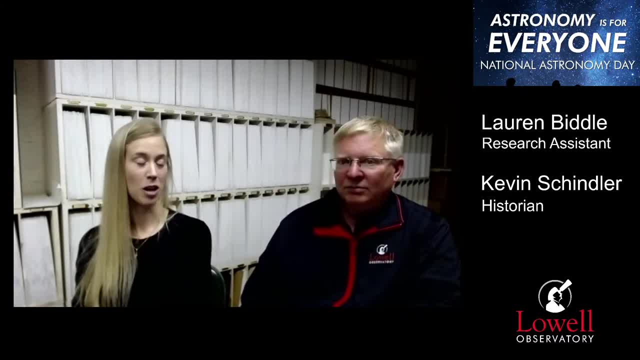 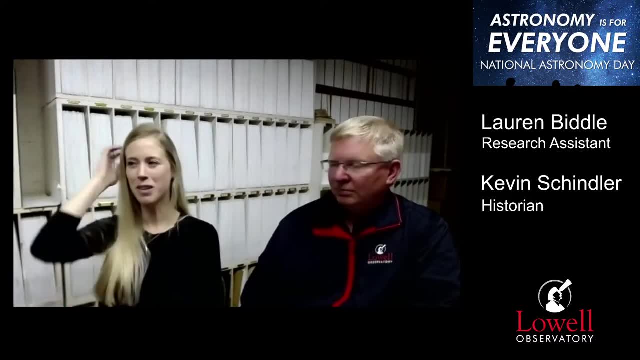 Bigger for me, I realized: oh, there's a lot more out there. I'm like actually seeing This object With my eyes, Not just like a picture of it. you know. Still, I mean, I think those are still beautiful and extremely inspiring. 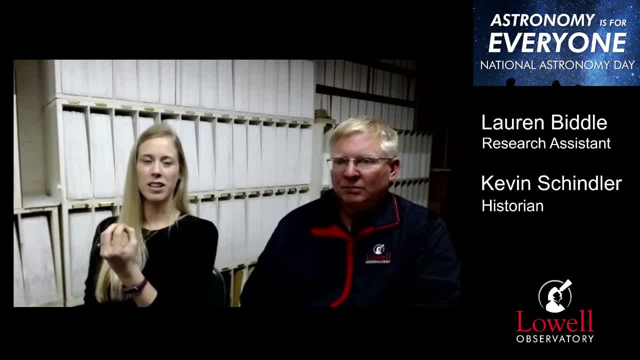 When you see them with your eyes, it's like You're. there's much more of a connection with it, I would say. And then my other favorite was when I was an undergrad at the university of Arizona. Yeah, It was my very first observing run. 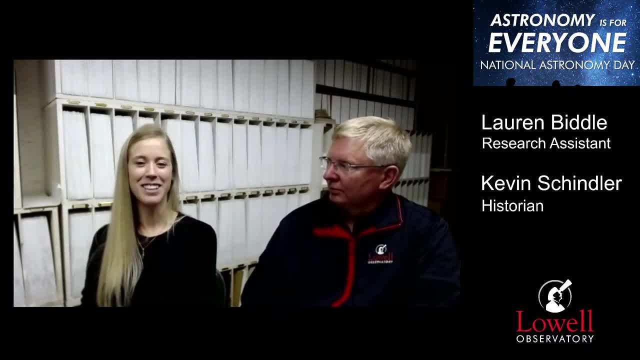 I went with the astronomer Betsy green. She took undergrads up to Mount Bigelow 61 inch telescope And we observed All night. It was a binary system We were looking at Just like, Just like planets, transit stars. 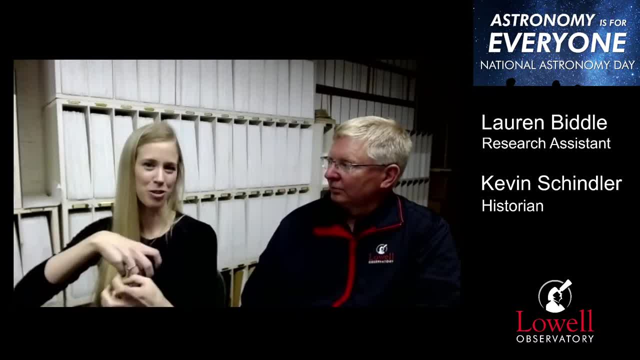 Other stars and binary systems can also pass in front of other stars, And so That's what we were observing: Just A change in brightness from two different stars- Yeah, Orbiting each other, and We didn't sleep all night. We stayed up all night and I was so tired. but 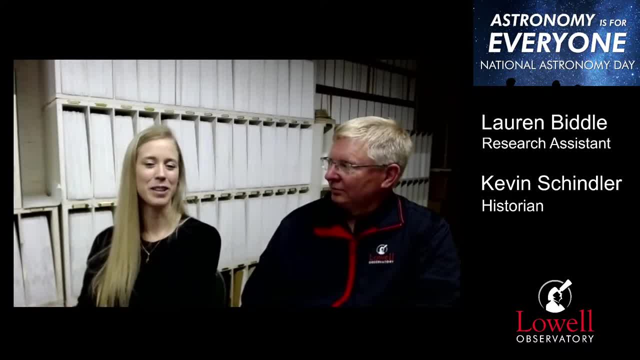 We got to watch the sunrise And we had the most beautiful view And I remember that was when I was thinking to myself like I knew I wanted to be a strong in astronomer. you know, I was in the program and I was. 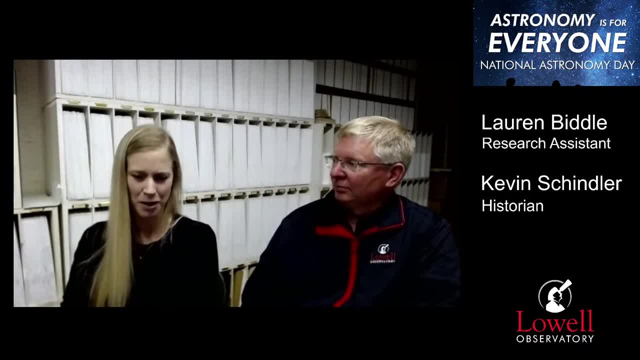 You know, doing the thing: doing my homework going home, Doing my homework going to class. But In that moment I realized, ah, I can do this. I could do this for the rest of my life. This is what I want. 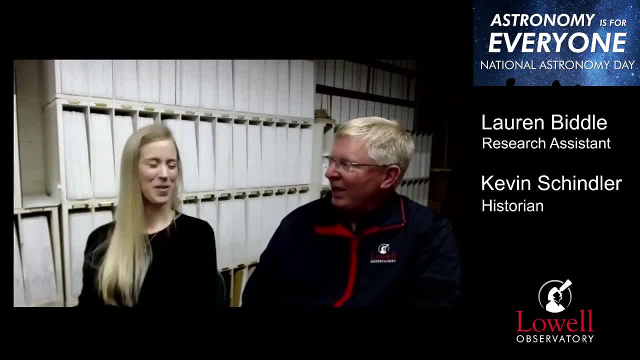 This is This is it? So I think that's the, That's magical, Yeah, And you know, it seems like Just about everybody you talk to. It doesn't have to be science, But people who have really followed their passion. There was something that fired them. You know Phil Massey, one of the scientists here. He went to He said it was a great experience And he said It's just about all. it's not all of the Apollo launches. Sending humans into space And that really inspired him and in some of our other scientists It seems like You know my interest is in science Goes to seven years old picking up a fossil They can might get. Look at this thing. And it just, it just captures you And it's that that magical age. It seems like I know the seven, eight, nine years old. yeah, you're brand new in it. you know you want to take it all in and it's interesting because you. 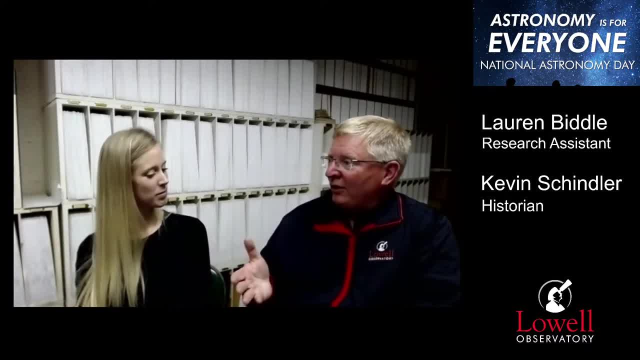 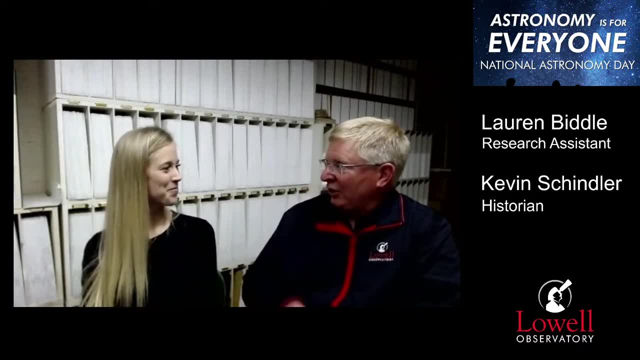 said: you know what those two things? um, one of them was looking through the eyepiece of a telescope with papa and the other was looking, probably at a computer screen, at the graphs of the of the brightness. is that right? yeah, all night. that's what we were looking at. we actually didn't even. 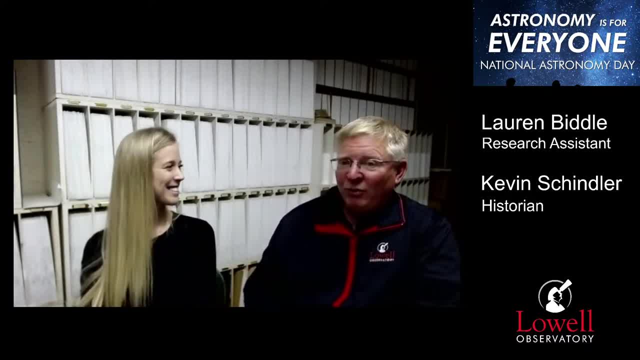 look through the eyepiece at all, and yet, and yet that's still because you, you realize what that means. um, you're, because it's not just looking at numbers or a graph, but it's what it, what you're learning from it, and that i think that's an important thing, because a lot of times there's 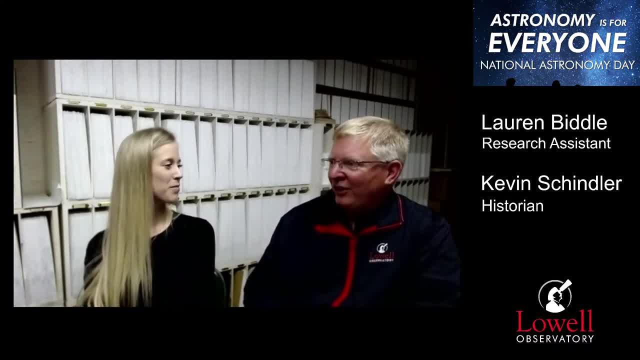 this idea of science, you know, staring at computers, looking at a bunch of numbers, but it's what's behind the numbers and and that's what you do is interpret it and then explain that to non-experts of what it all means. it's still very meaningful, yeah. 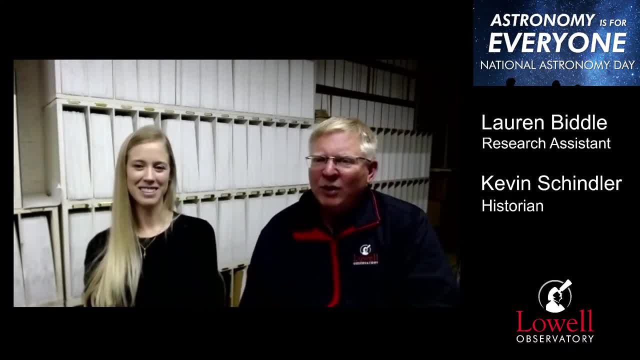 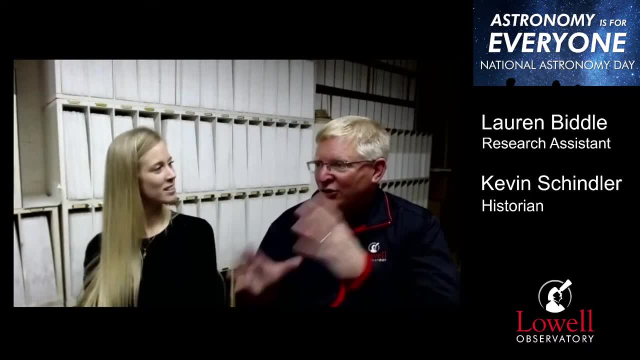 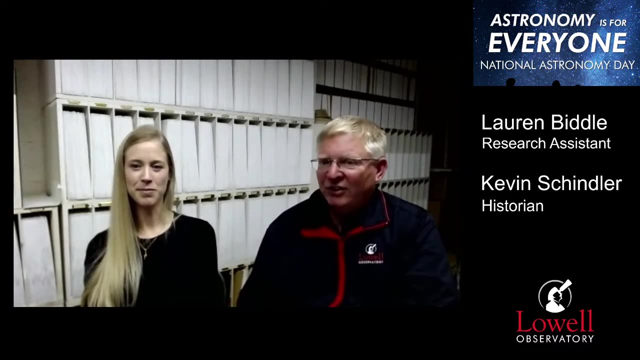 yeah, well, looks like we have about five more minutes so and i think we have a couple more questions. i'm kind of following up on your um discussion about your, your dream instrument, the interferometer in space. um, the question is, could you put telescopes or some sort of sensors on? 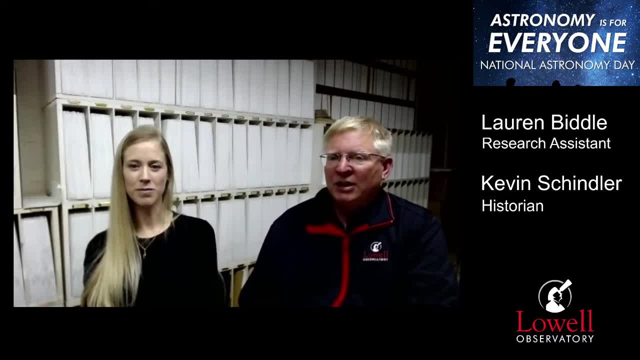 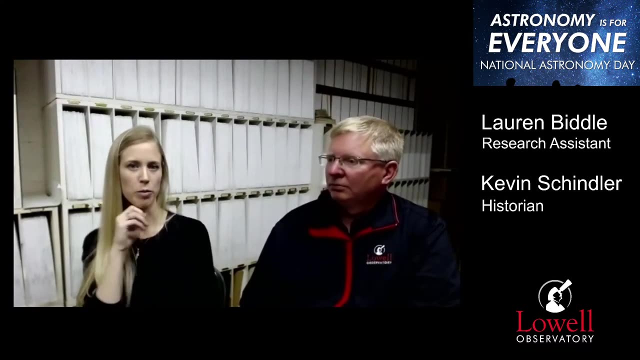 planets, the moon and um triangulate and have a you know, i mean that's kind of like a big interferometry system. yeah, i think, um, if we put them on different bodies, that might make it difficult, because those are would be, they would be moving constantly relative to one another. um, i've never considered something like that and i 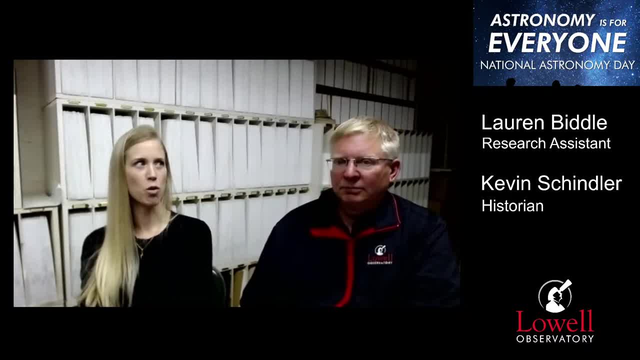 wouldn't write it off necessarily, um, but it would definitely take some more thought. i uh, yeah, some more thought and some more time to think about it than i think that we have. but, um, very, that's an interesting idea, yeah, and, and you know that's, it's amazing how far we've come, because i know 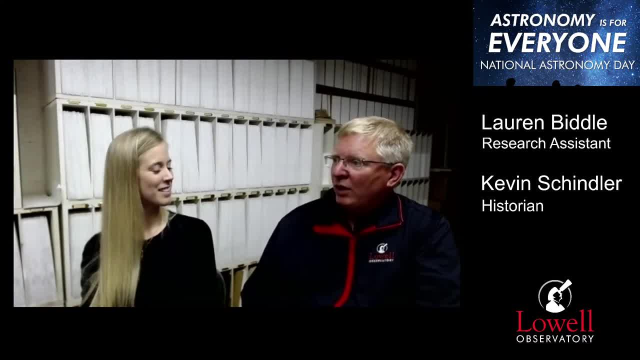 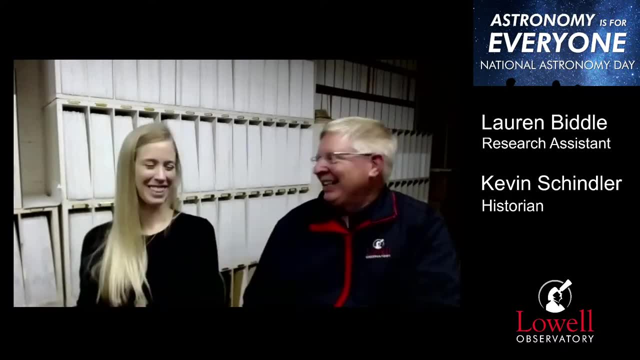 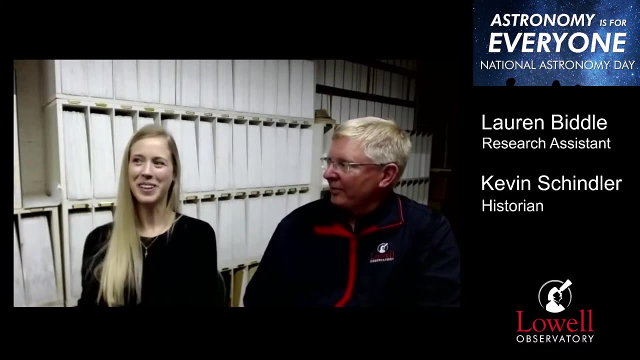 gerard van bell a couple years ago was working on a proposal um to do 3d printing in space. yes, i, yeah, well, i was actually at a conference. he gave a talk on that and um, the idea of building a telescope in space really um helps with uh, when you, when you make it in space 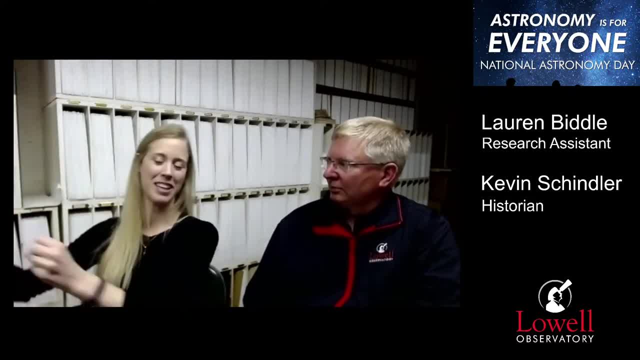 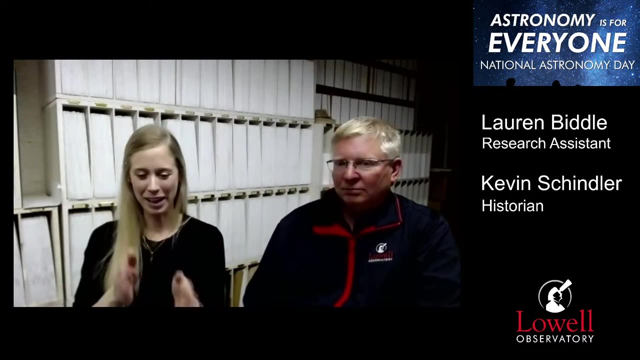 you don't have to send the whole thing up at once. it's not as heavy, and then it also allows you to do some things that you wouldn't have been able to do: um here and then get it up there. um, that's just like the the right away benefit to that. but also when i was talking about, like my 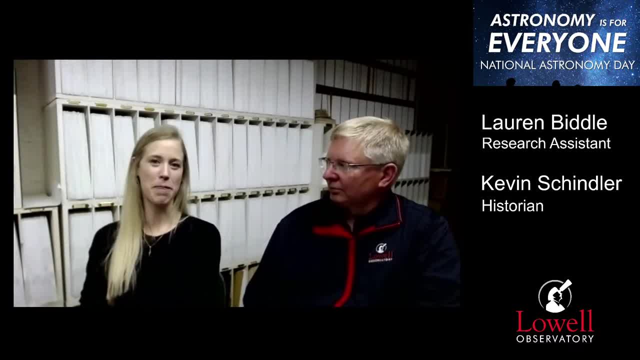 dream telescope that, like wide interferometer, um, his proposed um instrument, would actually allow us to image the young star systems that we look at. and so i'm, i'm all for it, i, i'm behind him 100, and it's only a matter of time. i mean, we start. 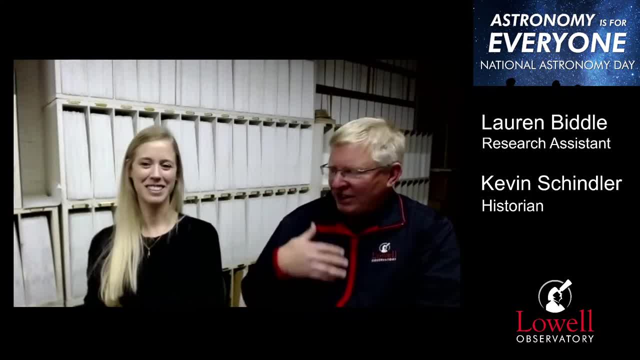 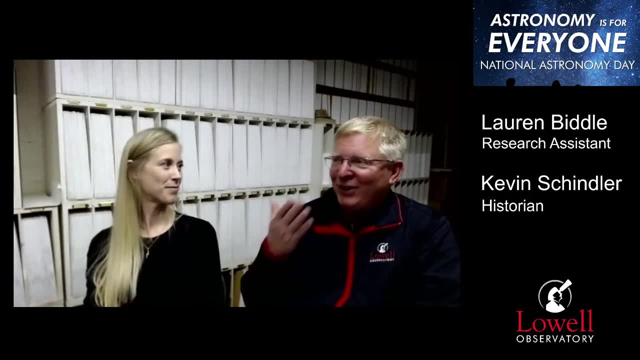 getting these ideas. like all science, you get an idea and it sometimes it takes a little time to develop it and the technology. but you know, 3d printing is changing how we do a lot of things and to think you can build, you know instead of instead of assembling it here and then getting. 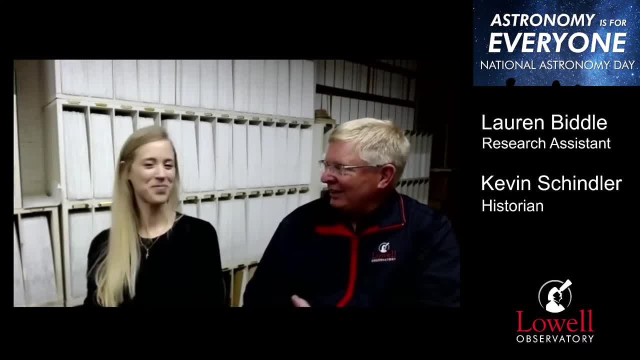 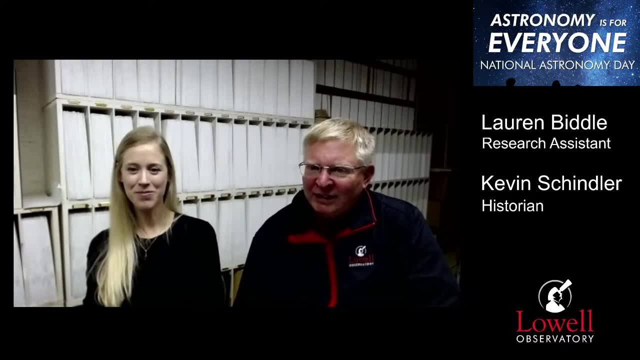 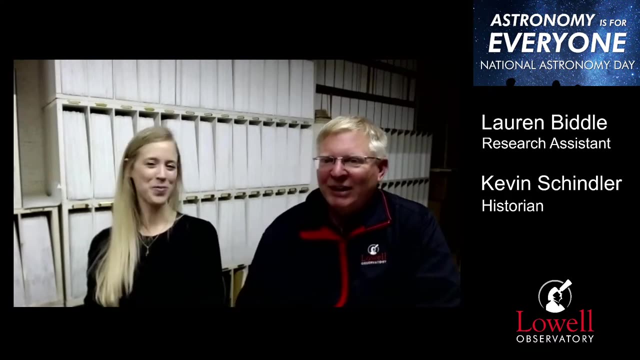 it up there, building it in space. it's hard to imagine yet that's going to happen. it's so neat. well, we've got just a couple minutes left here. um, so let's go through the last comments and if anybody has any final questions for the future, dr biddle, um, write those in in the next couple minutes. 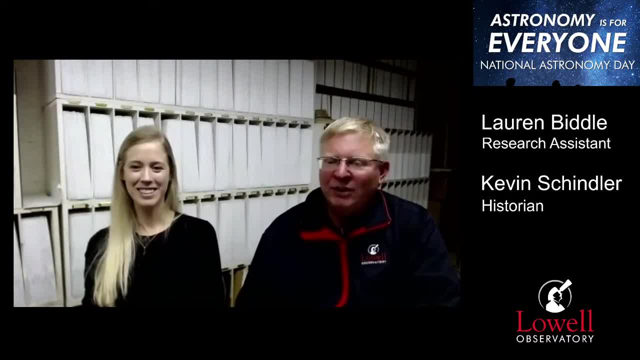 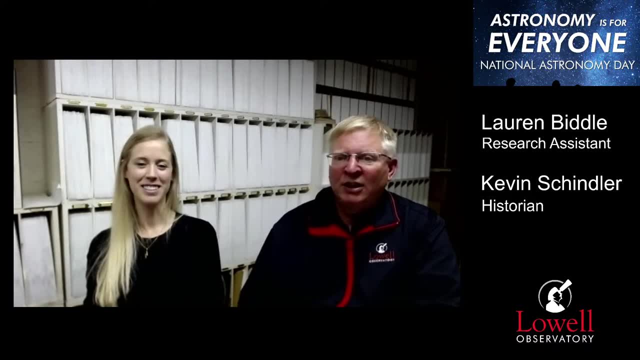 um david moore, was david? you're going to be visiting flagstaff um, so i'd be. i'd love to talk to you um. i'm kevin at lowelledu, my email kevin at lowelledu, so get a hold of me and we'd be. 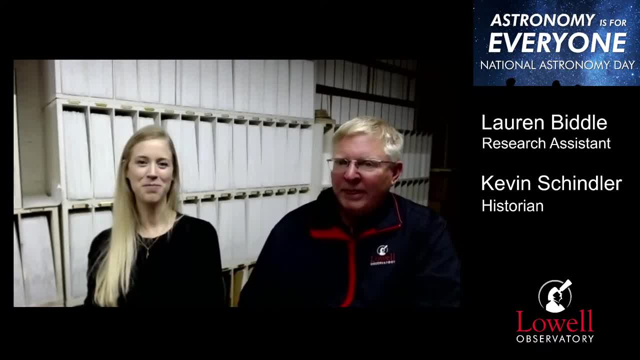 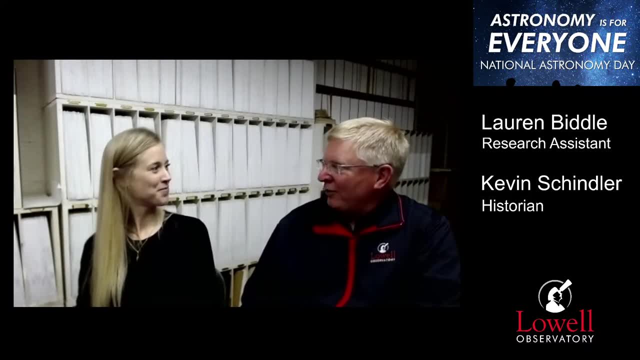 glad to um talk to you, look at some pictures and everything, and i'll see you next time. um, so let's, we've got just a couple minutes left. so let's see, i don't know, 35, 40 years from now, you're going to be thinking about retiring, maybe, and as you look back on your career,